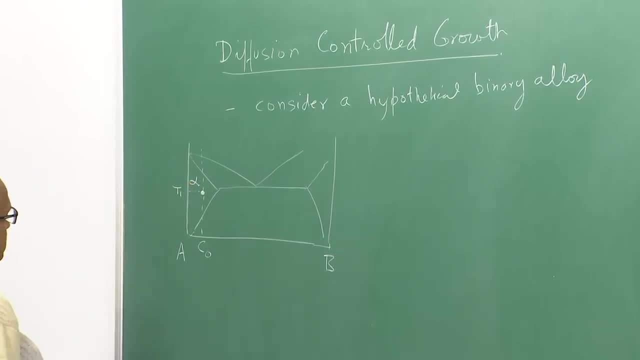 alpha. Now imagine that we suddenly bring the temperature down to some temperature T. So we are at this point and we are now in the two phase alpha plus Cd. So we have two phases alpha and we have two phases T. So we have two phase alpha and we are in the two phase, phase T. 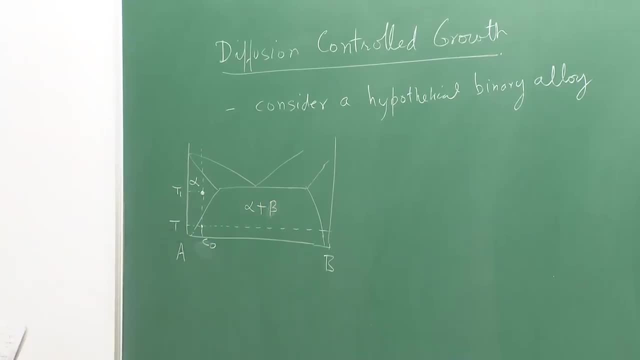 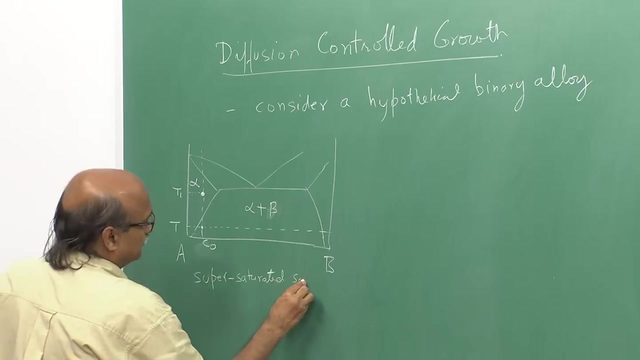 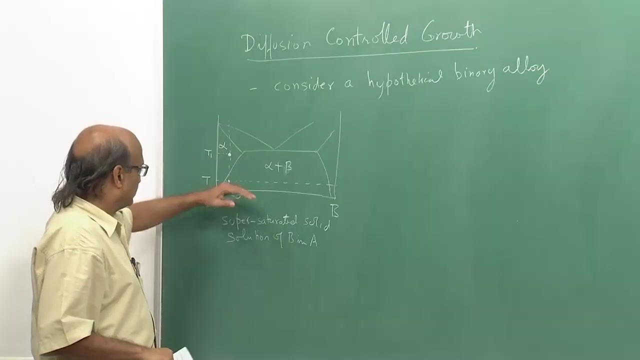 beta region. So what we have now is a super saturated solid solution of B in A, and hence this super saturated solid solution will tend to break and beta nuclei will form at this temperature T, and once a stable nucleus form, that phase will tend to grow. then. 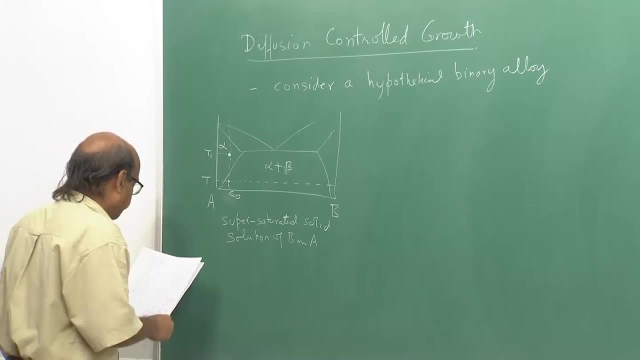 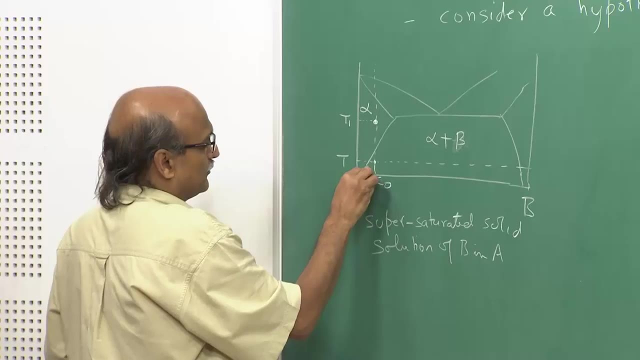 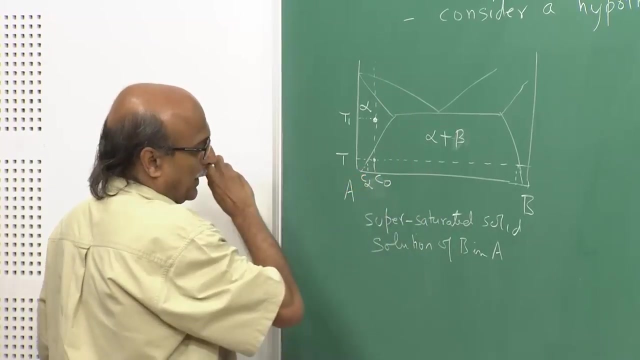 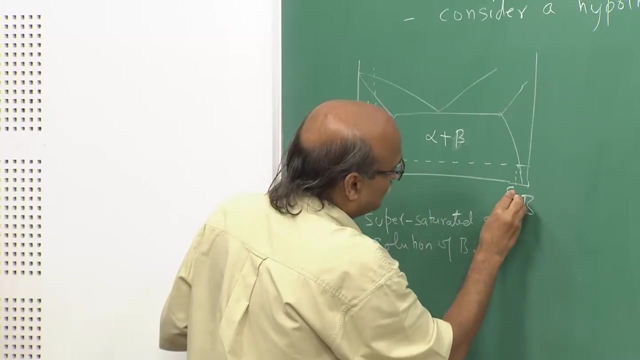 So beta precipitates B. This will grow and they should grow. if you look at the equilibrium that is required, the alpha should have a composition of C alpha and the beta should have beta precipitate. that forms should have a composition of C beta according to this phase diagram. So 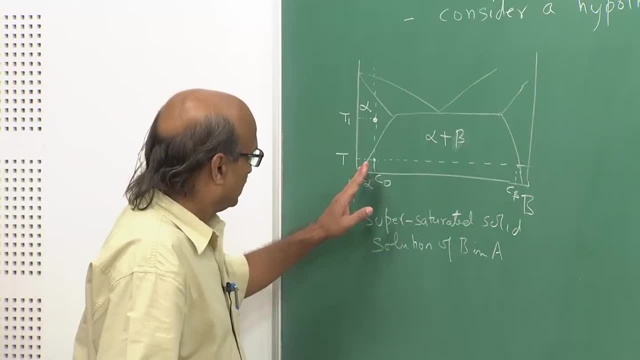 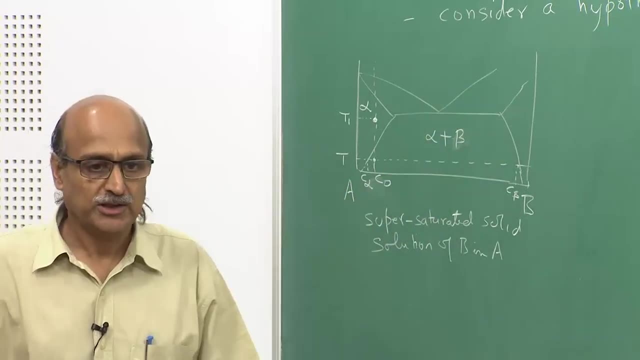 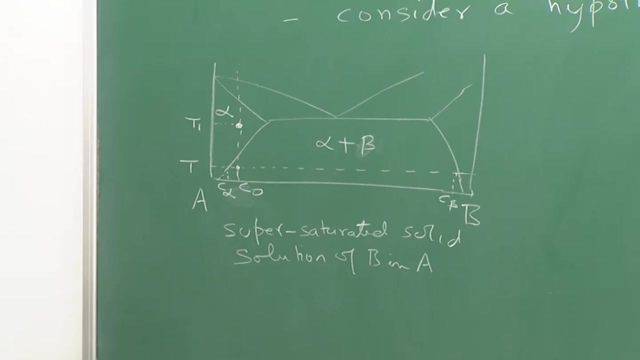 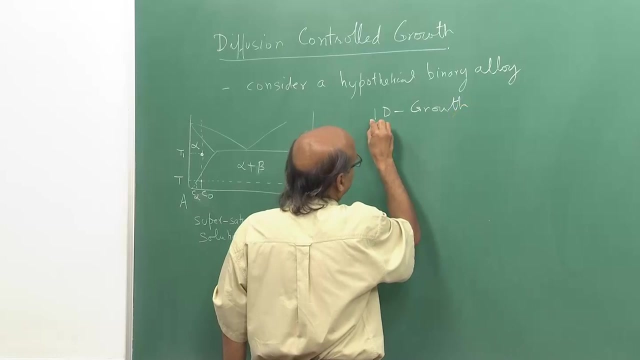 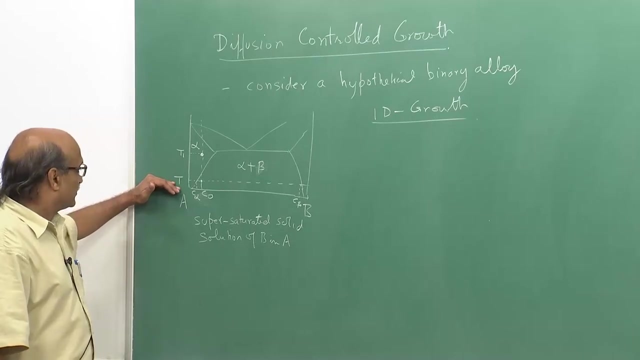 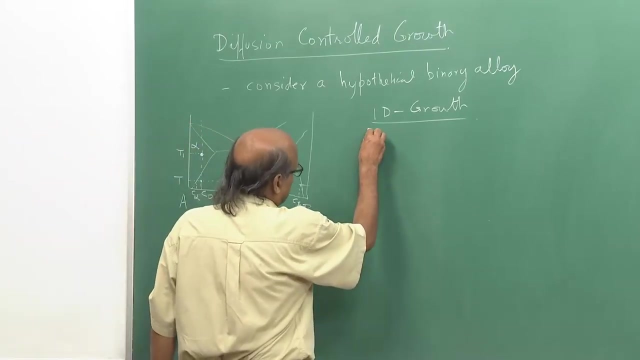 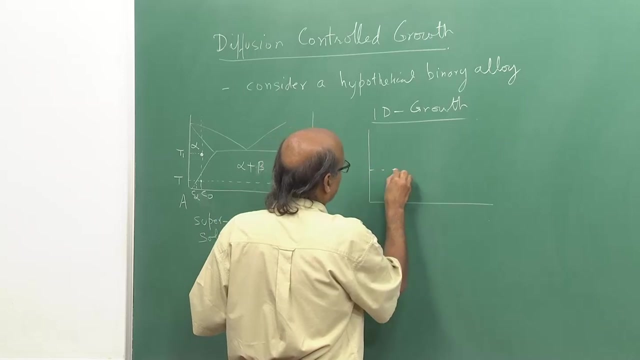 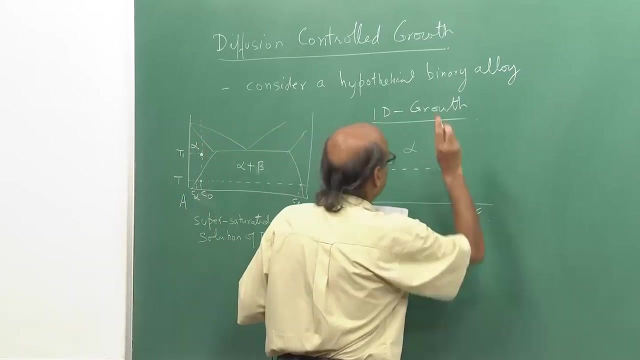 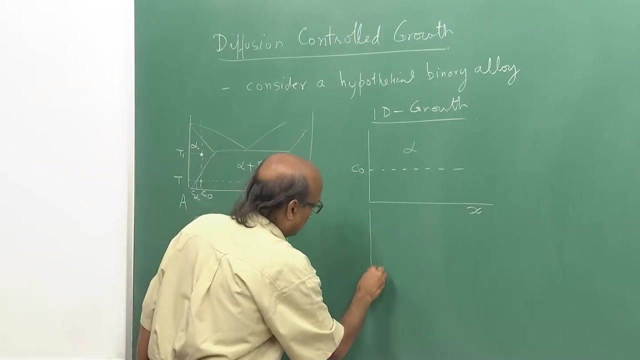 this C alpha. We quench it from T 1 to T, So at time T is equal to 0. all one has is composition C naught, and we have only the alpha phase, but as a nucleus forms and then it starts to grow. 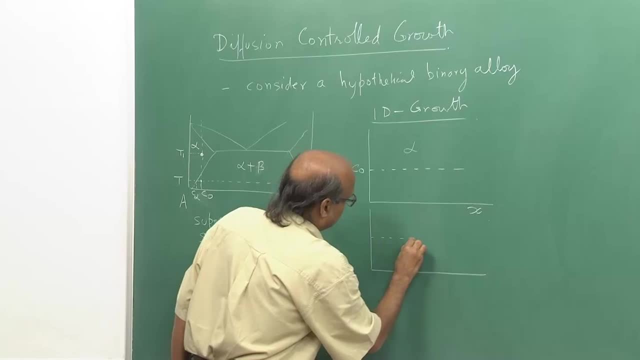 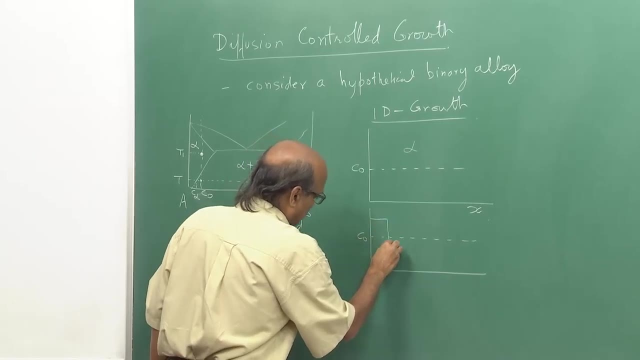 So I will do the initial, though this is the initial process and we do the initial process here. So this is the initial process. So we have a picture like this. So I have C naught here. I have, let us say, a slab of beta that is formed. So I have 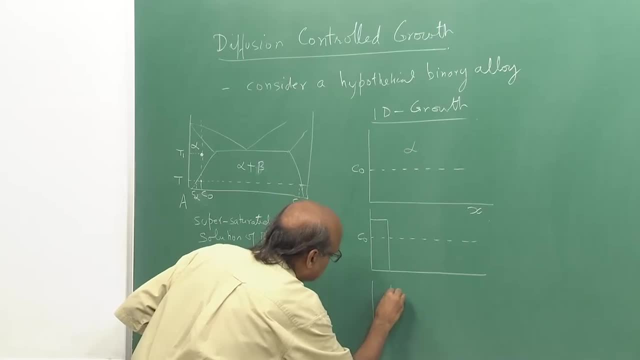 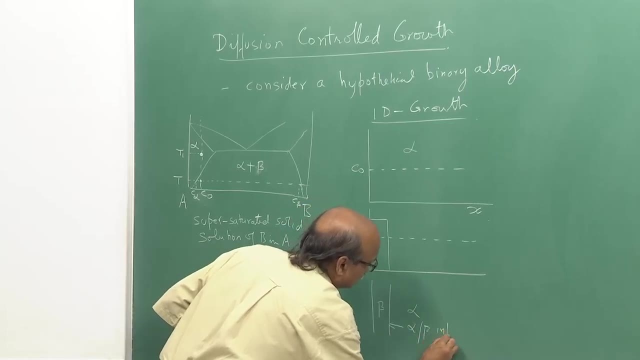 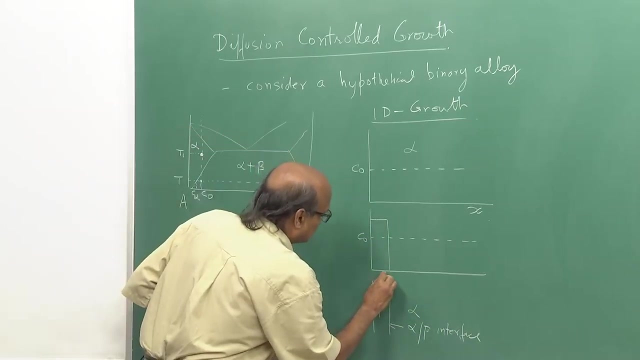 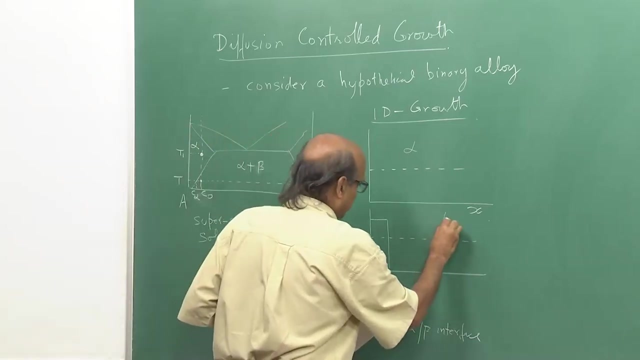 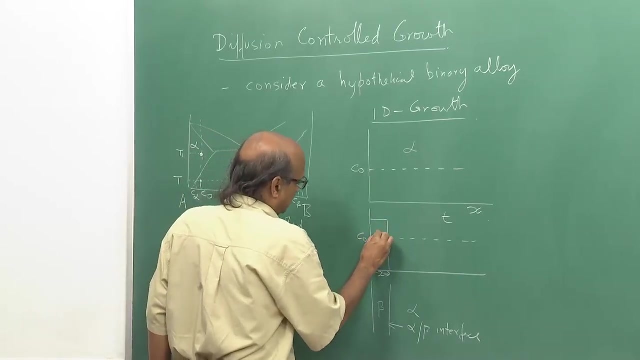 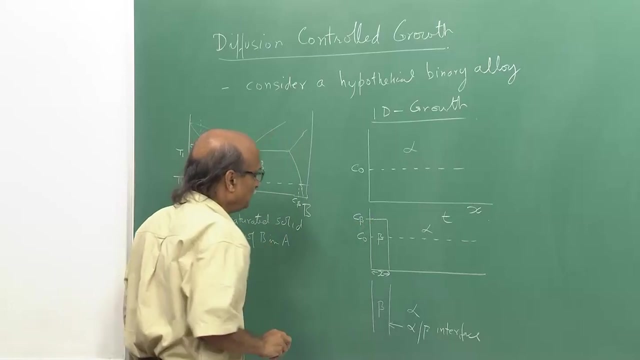 a slab. imagine situation like this: this is my beta, this is my alpha. this is my alpha beta Interesting, right, Yes, interface, and this is of thickness x and this is, at some time, t, this composition of the beta that forms. So this is beta, out, here is alpha. this composition is c beta, the equilibrium. 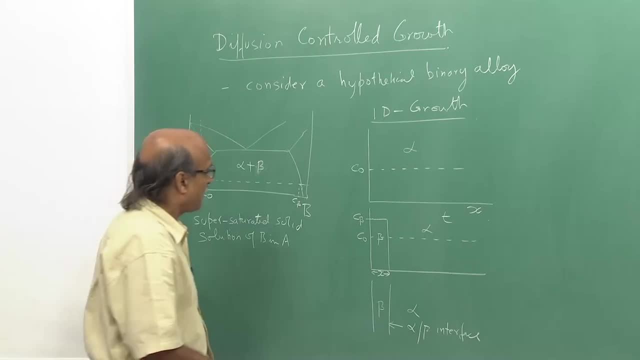 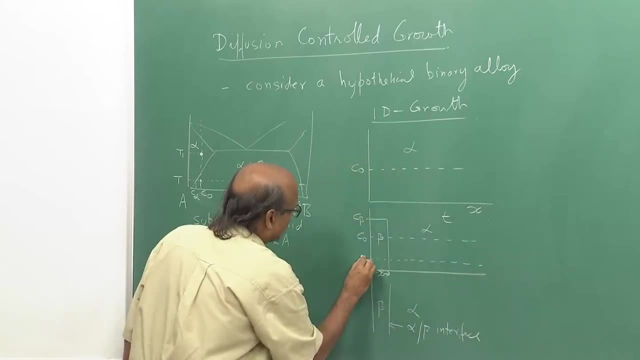 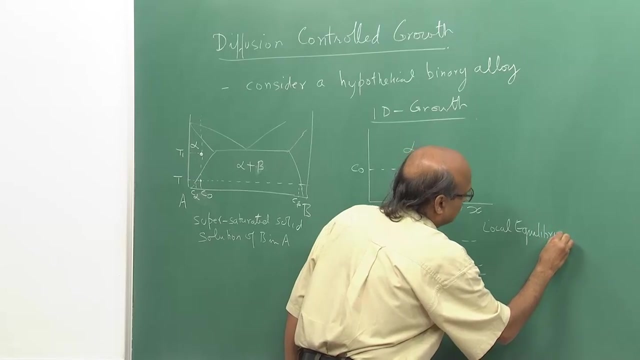 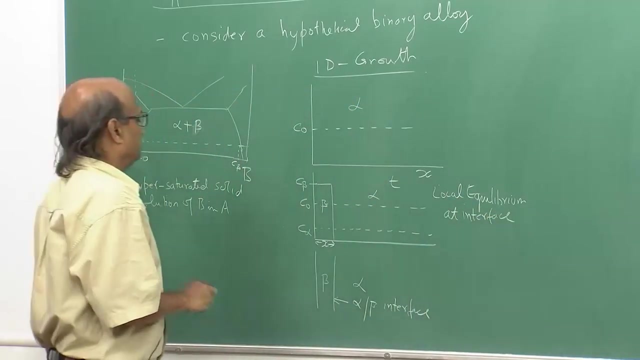 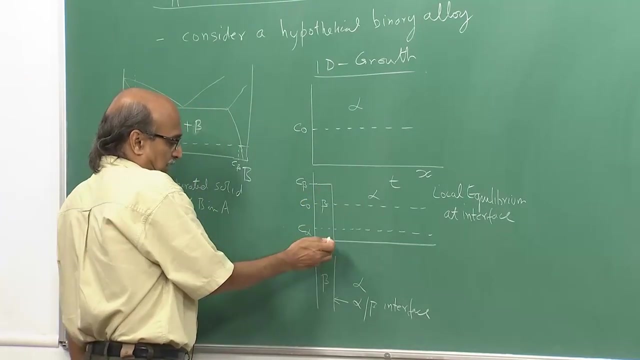 composition from the phase diagram. and let me mark the equilibrium composition for alpha here. So let us assume local equilibrium at the interface. If you assume local interface at the interface, what does this mean? that in this? 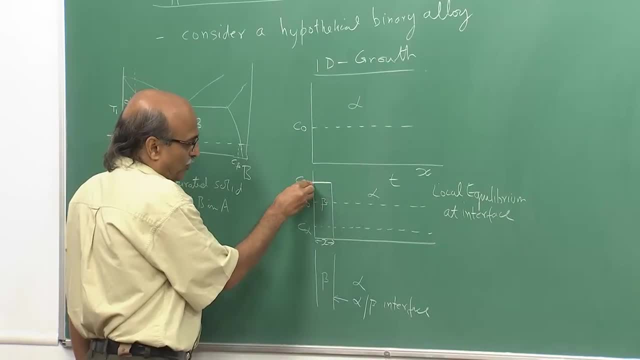 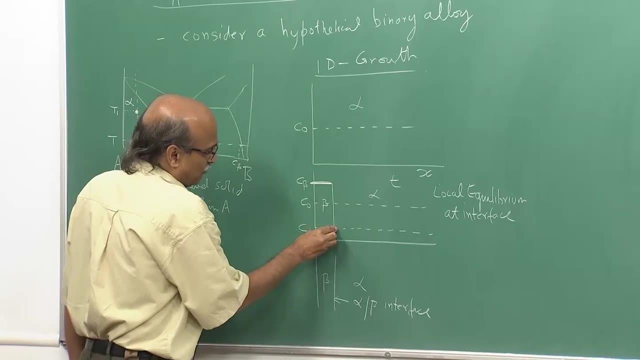 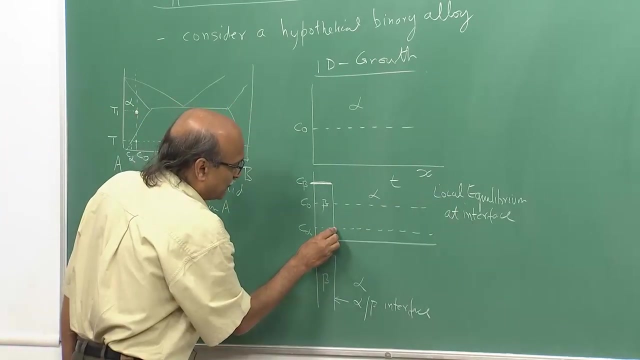 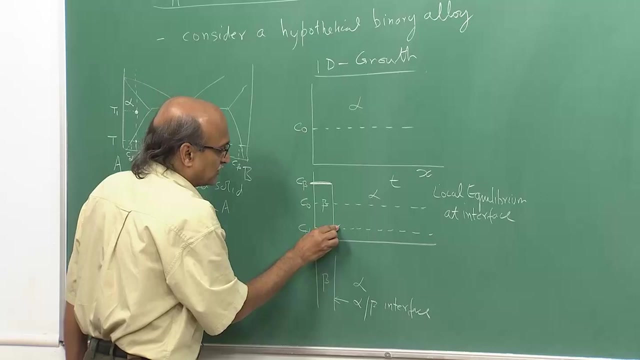 region, the beta would have the equilibrium composition of c beta and out here alpha, at the interface, would have a composition, equilibrium composition of c alpha and far away from this beta precipitate the composition will. in inside, alpha would be C naught, So hence the composition, or 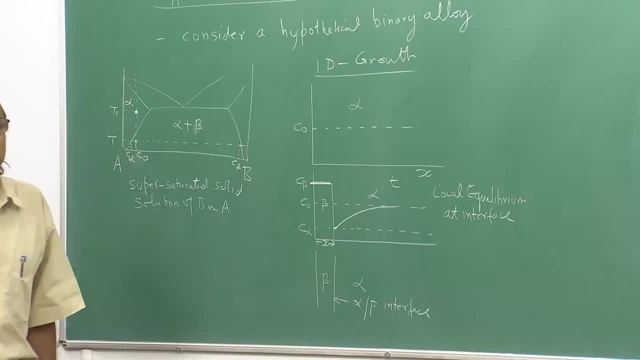 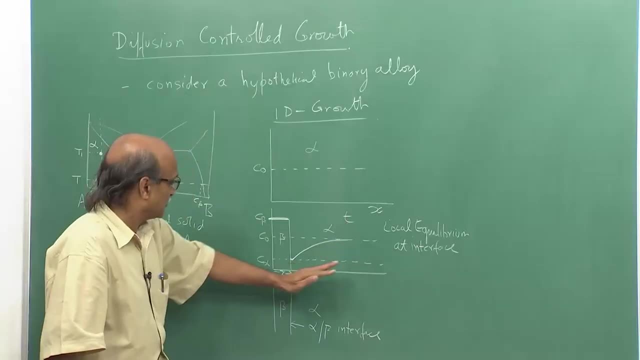 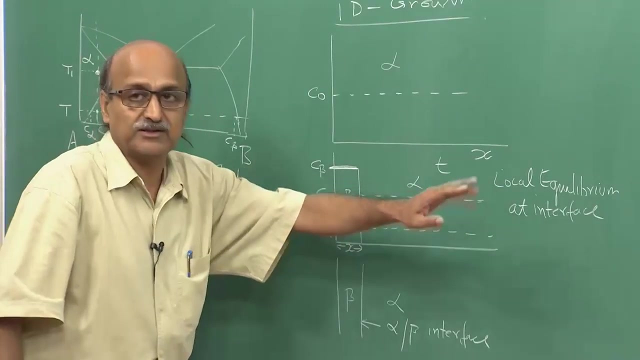 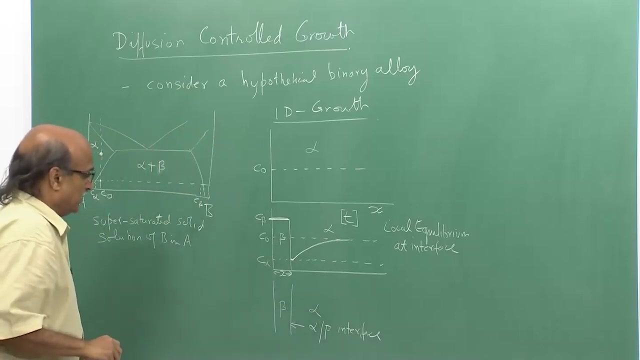 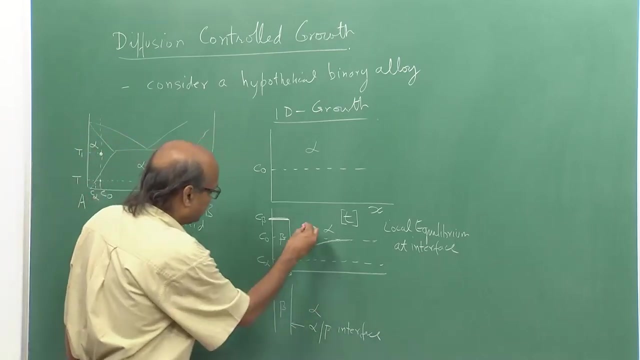 the concentration profile within the alpha would be something like this. So it will, as one moves into the alpha, away from the beta, precipitate. the concentration inside the alpha would increase and reach the starting alloy composition of C naught. This is at some time t Now, after an elapse of time d t. So this is at time t, at time d t this. 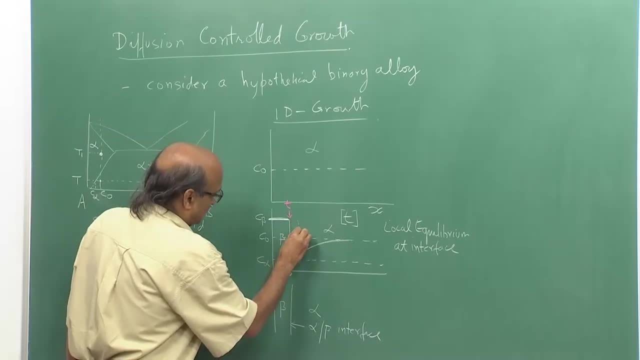 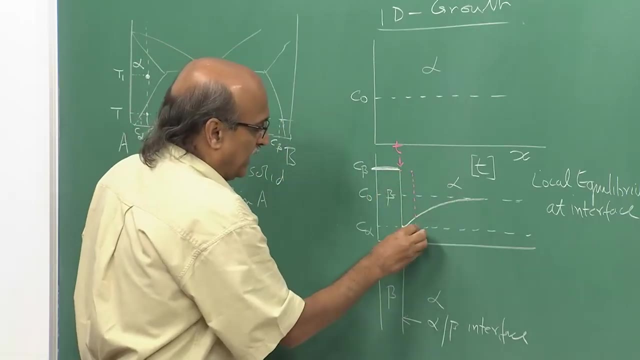 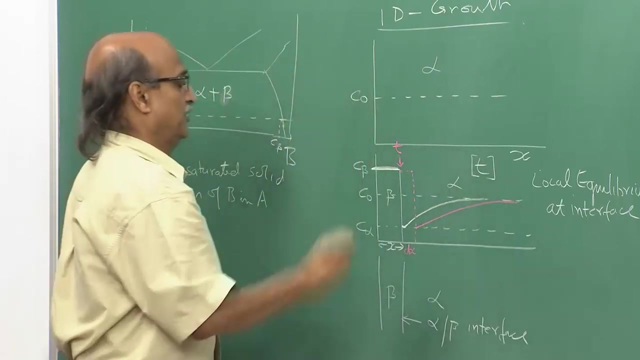 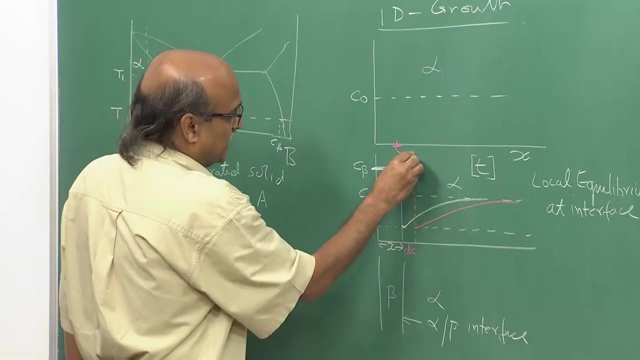 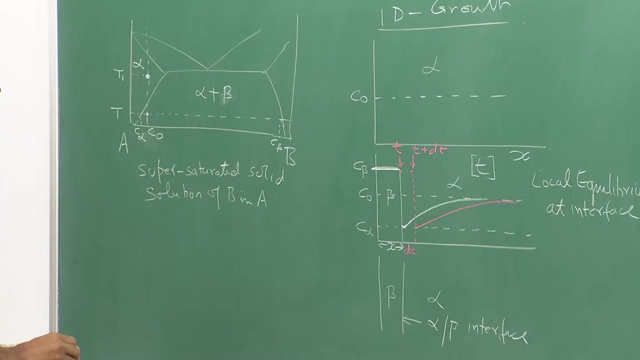 beta precipitate will grow by a, by an amount d x, and the composition profile in the alpha would also change like this. So this, so the interface at time t was here, interface at time t plus d: t has moved by a distance d x. So this is, this is the situation. 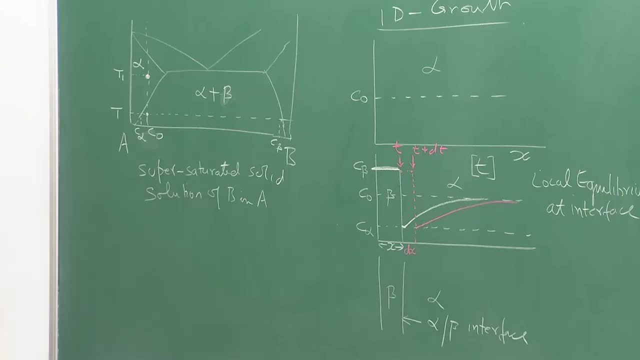 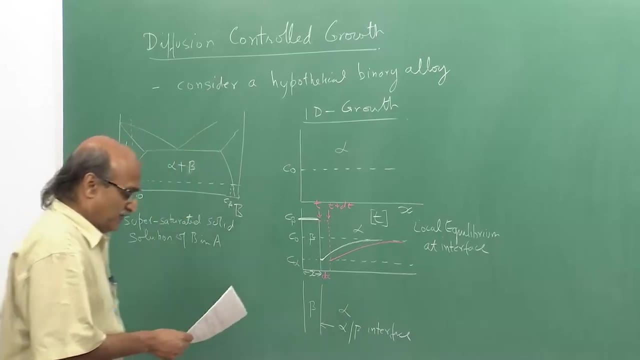 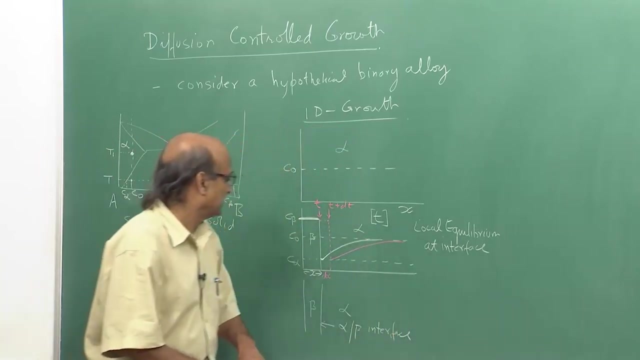 that we have Now in order to solve this in a, in a kind of a simplistic manner, just to show how, what is the growth kinetics in this, we make a, we make a small simplification, and the simplification is that, instead of assuming a curve profile like this, which actually 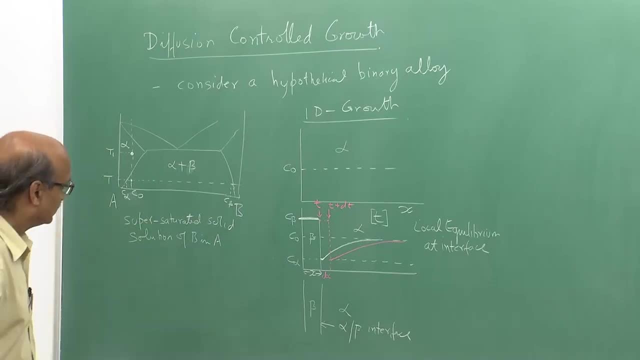 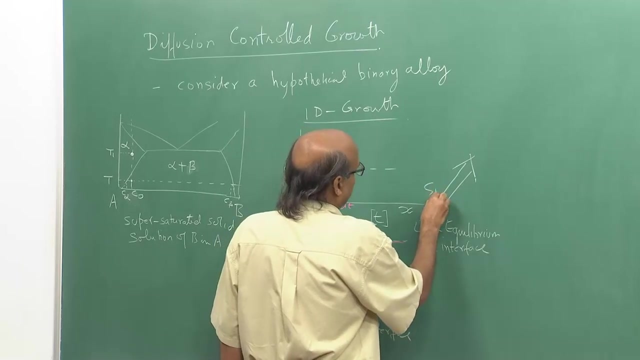 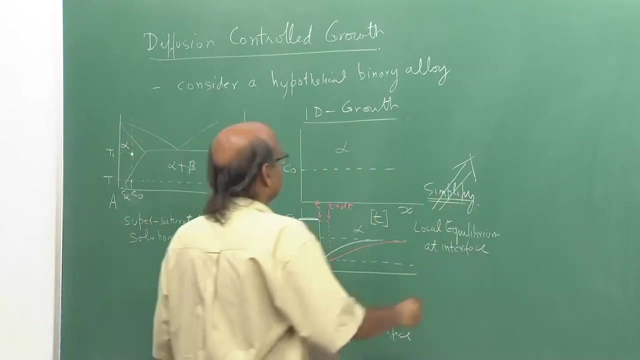 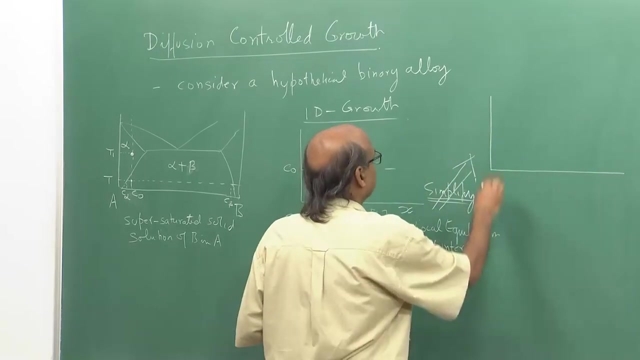 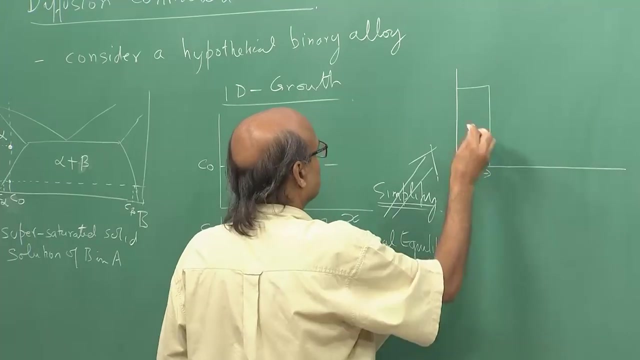 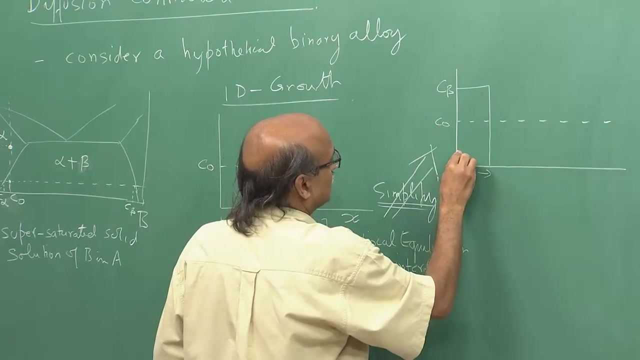 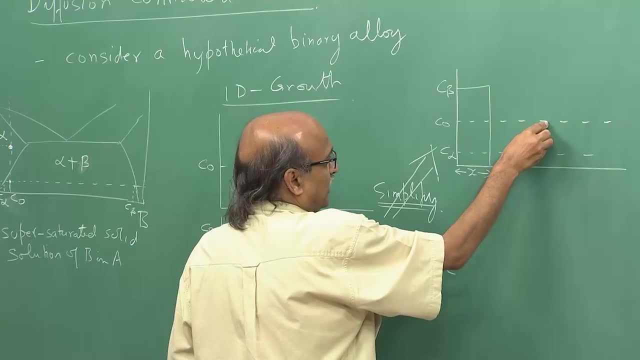 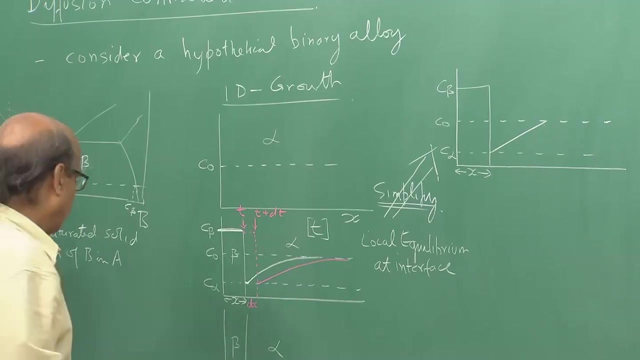 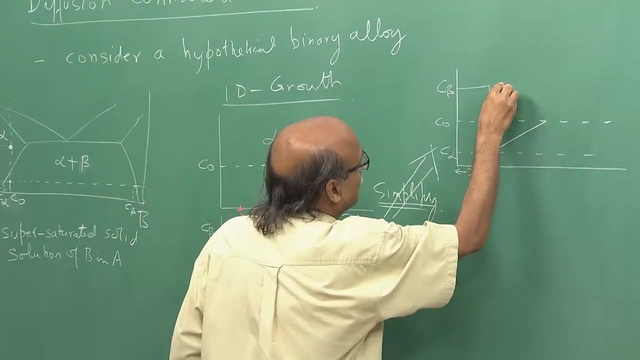 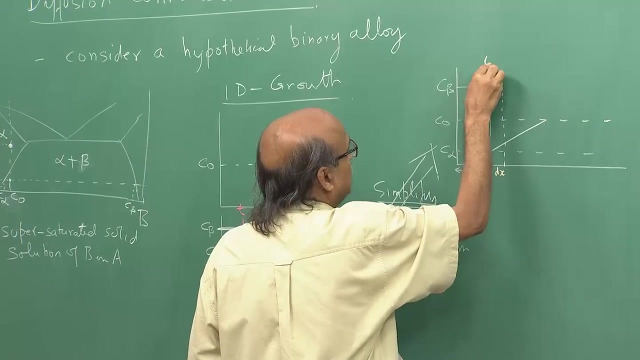 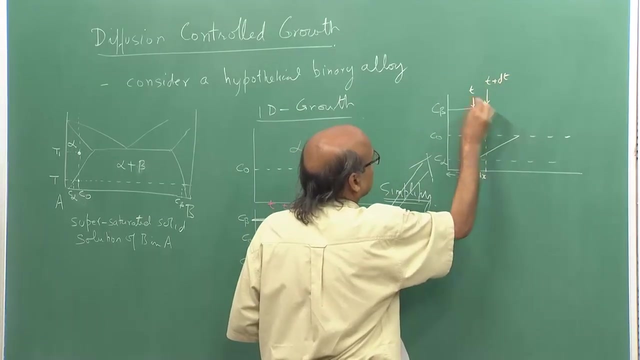 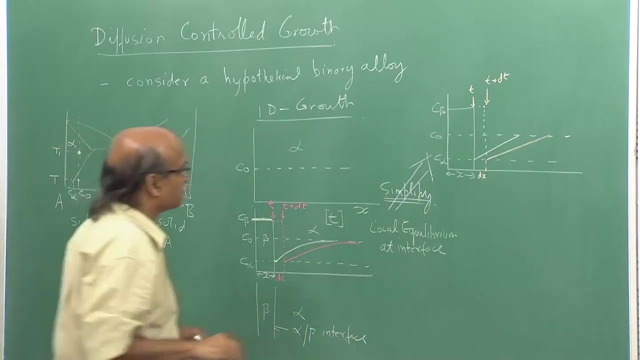 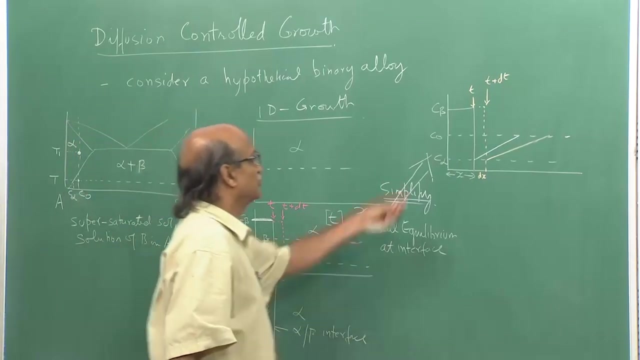 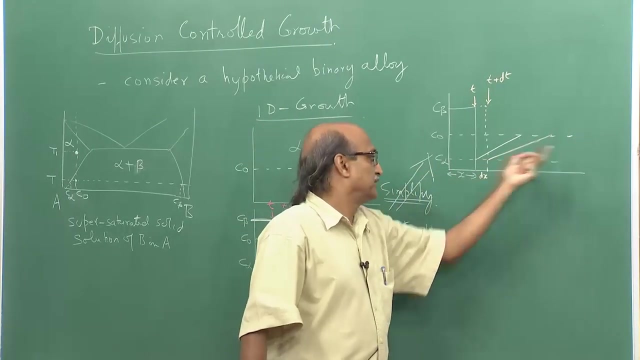 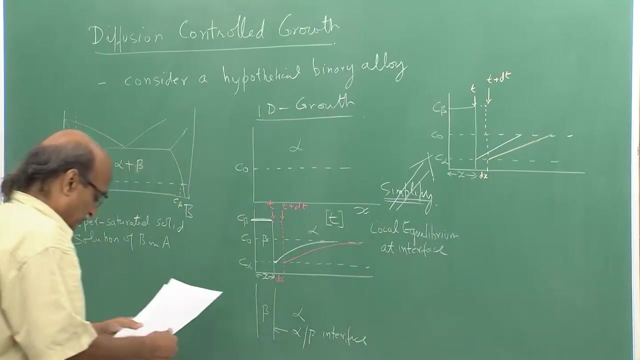 is given by a complex function called the error function. we assume this profile to be a straight line, So the velocity with which this interface will move and how the distance or the or the distance of the interface changes as a function of time. So the velocity of the interface. 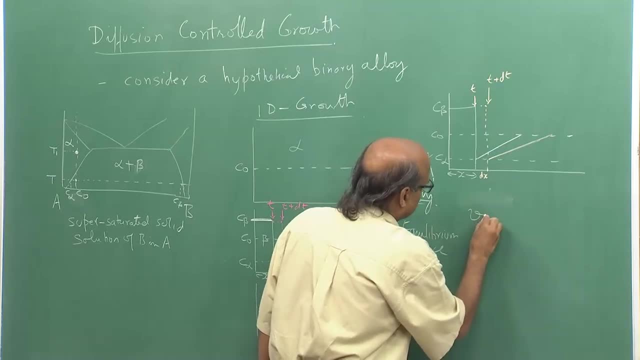 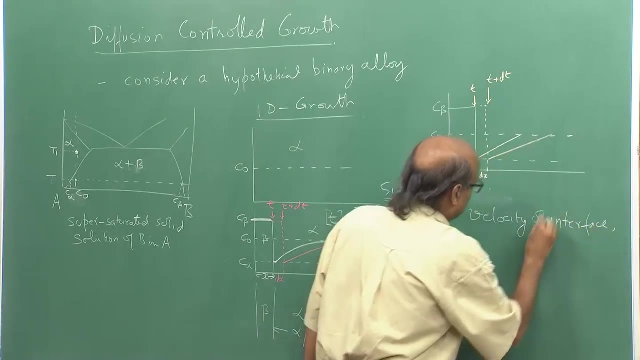 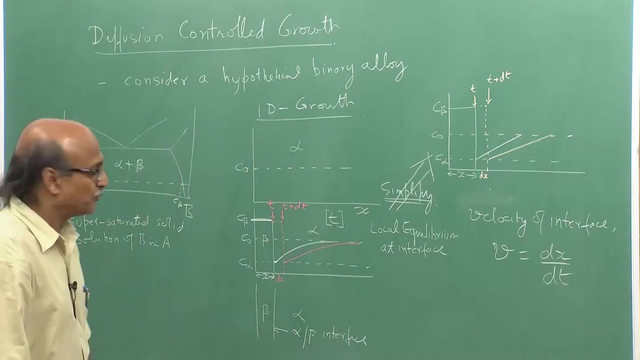 V is simply dx by dt. So our objective here is to find this that would give us the growth kinetics. So we will look at this simplified picture and attempt to solve this problem. Now what? 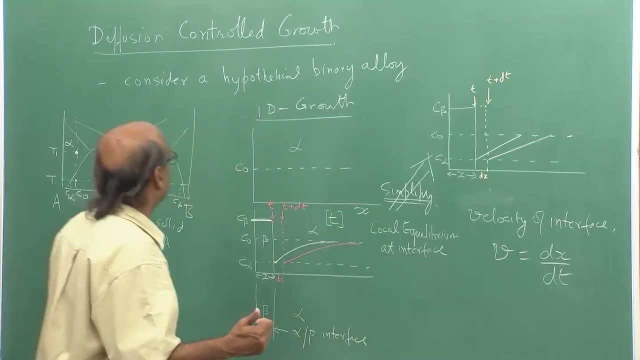 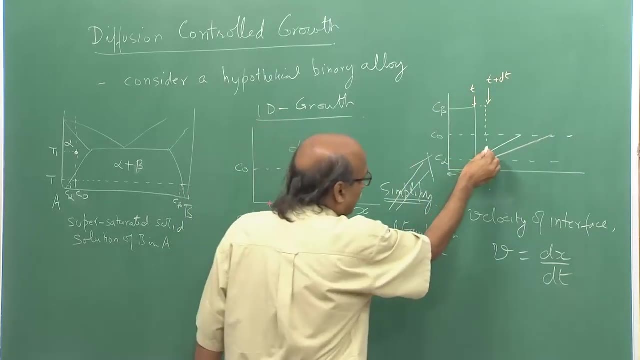 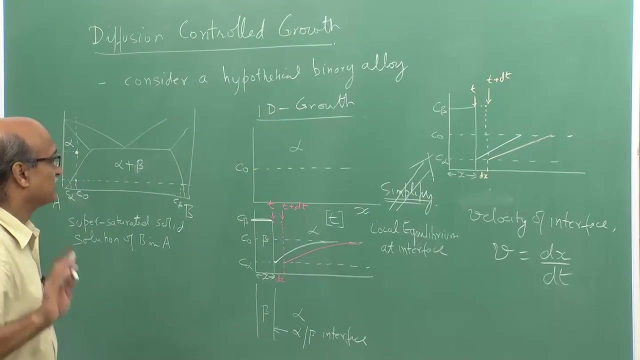 are the processes that are happening. Remember, this is diffusion controlled process that we are looking at So, and not interface control. So the jumping of atoms across the interface is a very fast process and therefore we can neglect it and the rate is essentially controlled. 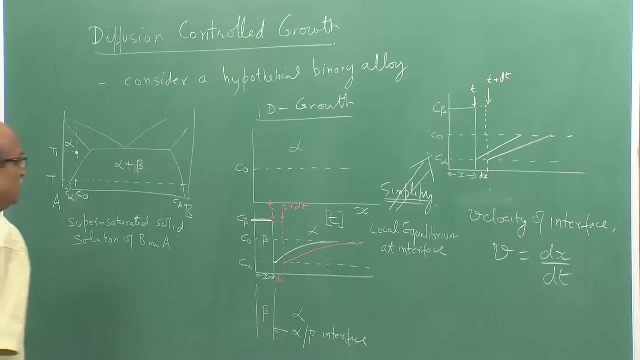 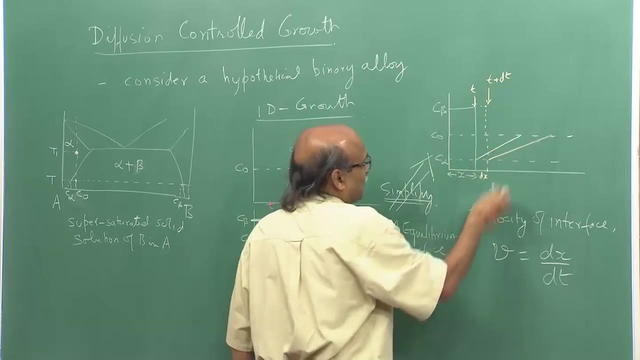 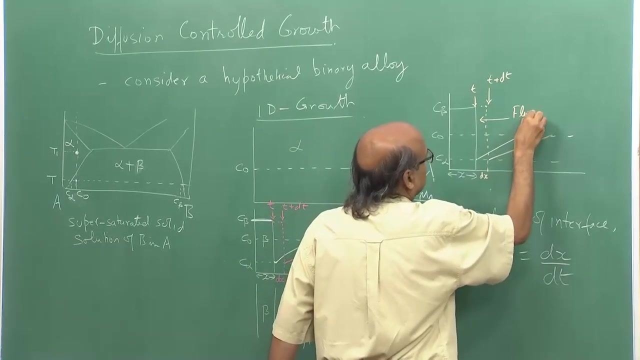 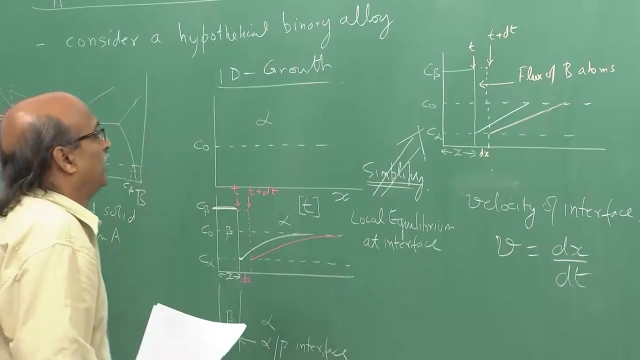 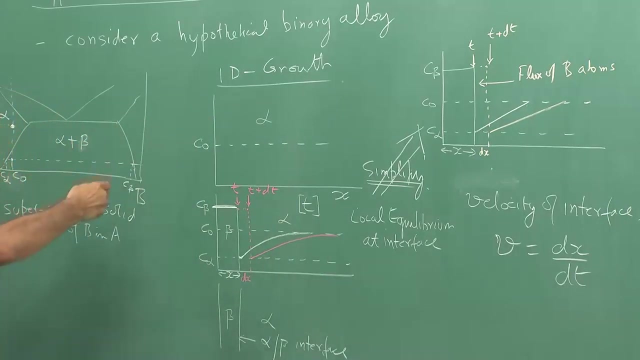 by the rate of diffusion of atoms. In this case one would need B atoms to diffuse, So there will have to be a flux of B atoms diffusing across the interface in order for this interface to grow or for this interface to move, or for 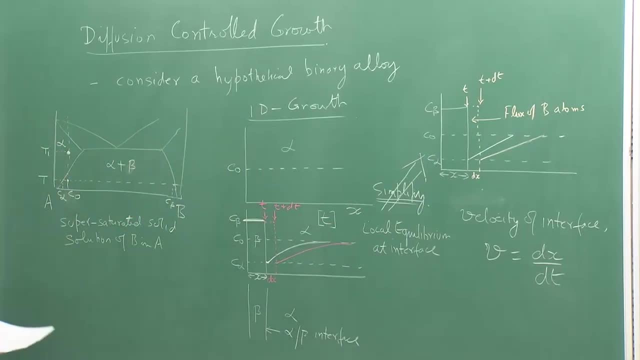 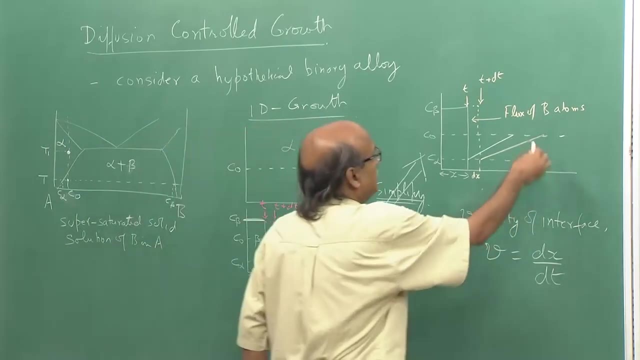 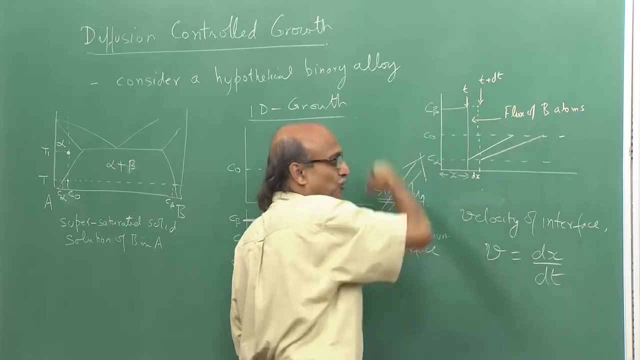 the precipitate to grow. So let us look at it. What is the flux of B atoms? At what rate can B atoms be diffused? By the way, the context is very simple. A flux of B. B atoms is a flow of B- slugs, material. 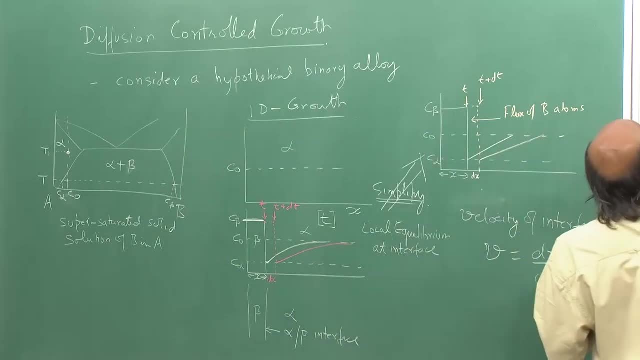 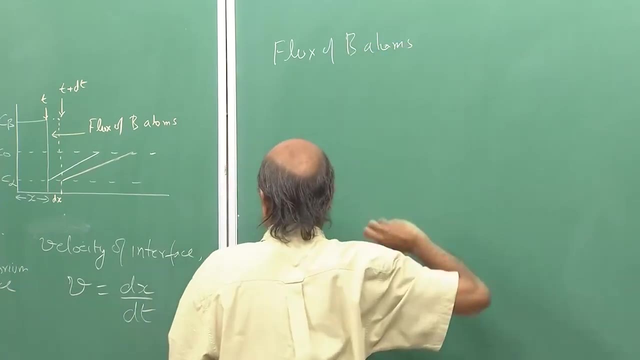 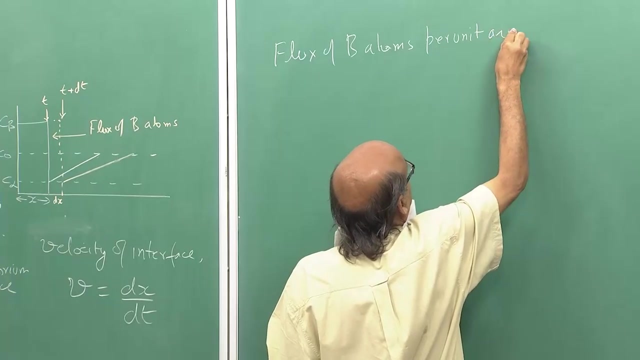 that was created in the form of muons in B plus for minus, muon for Gloucestertans And that flow is known asumentary flow. The slugs material according to the flow of B act, starting with muons, is a momentary flow of B ascent. And that is especially that the flux of B 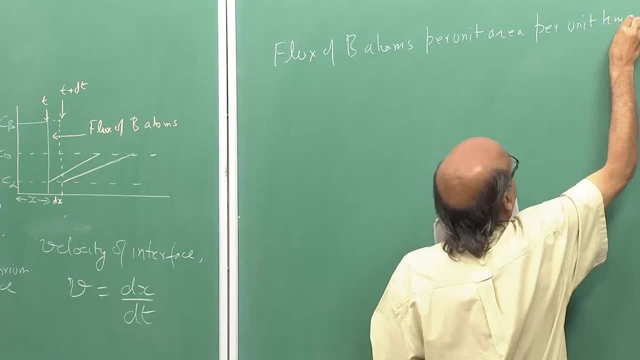 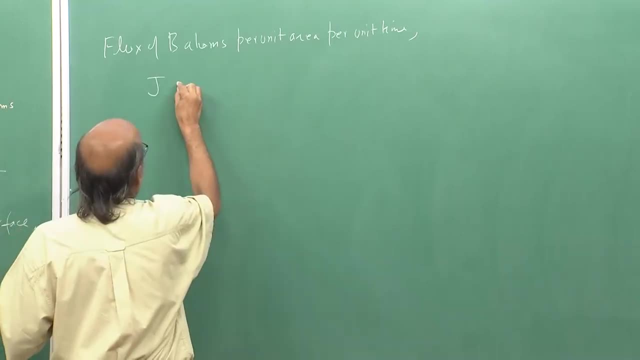 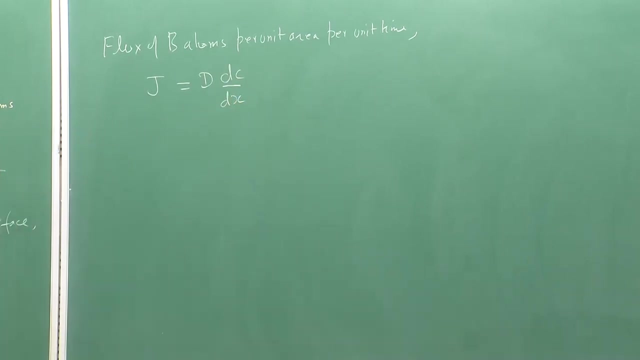 B Аs is similar to that of Z, So the flux of V is similar to that of B Alوسi, Vietnamese ascent. If I call that as J, then this is given by d, d, c, by d x. Now, what is this relation? 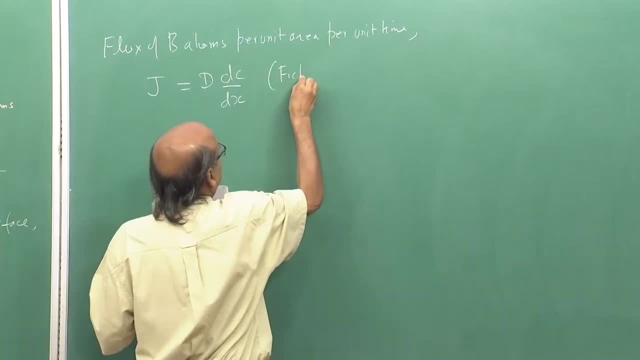 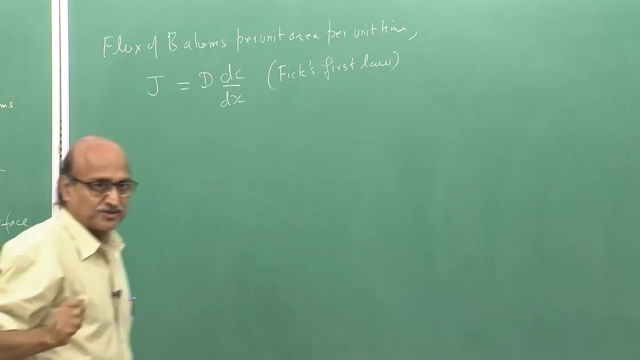 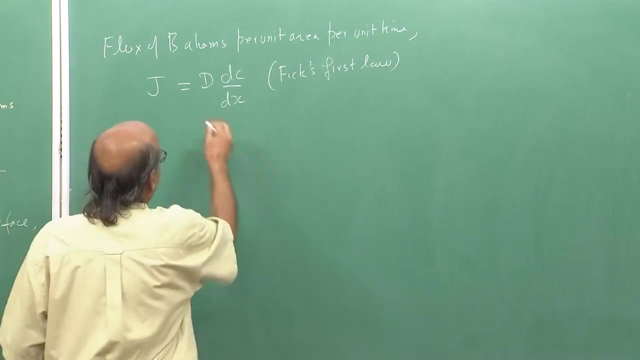 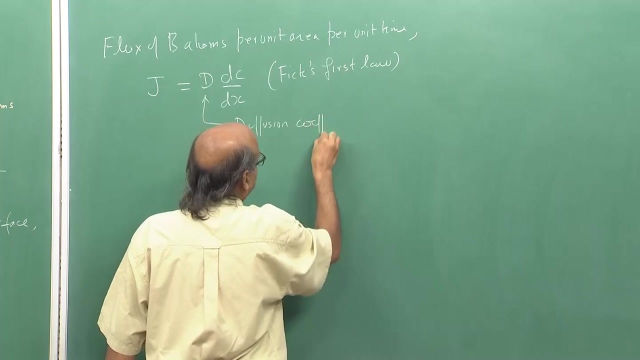 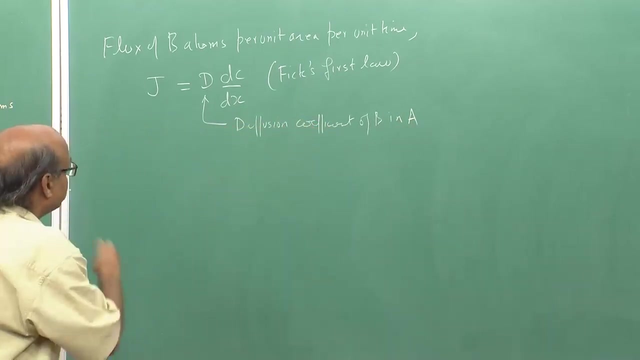 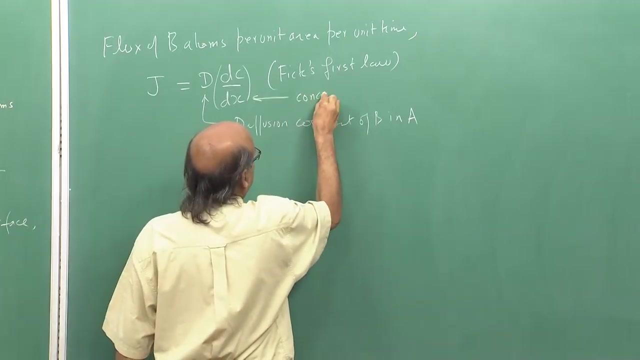 This, in fact, is called the Fick's first law, which we will be discussing in subsequent lectures. For now, let us take this relationship as it is. d is called in this case the diffusion coefficient of B in A, d, c by d. x is the concentration gradient. 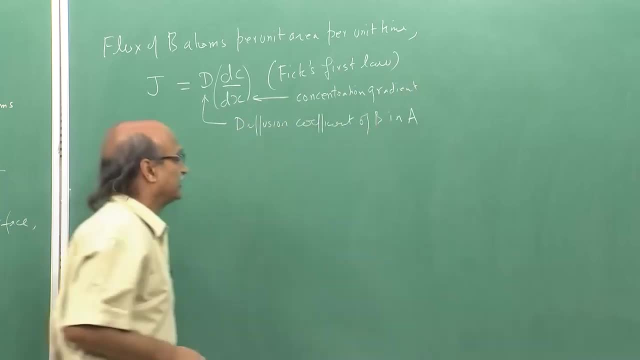 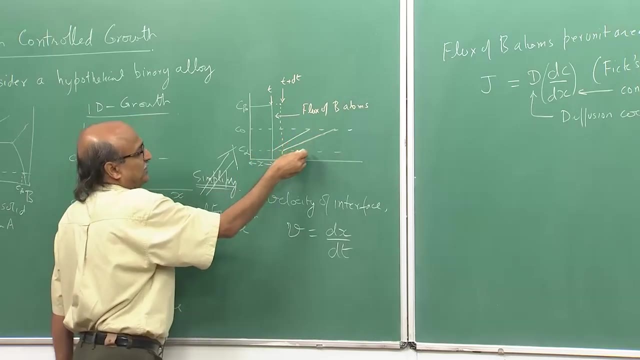 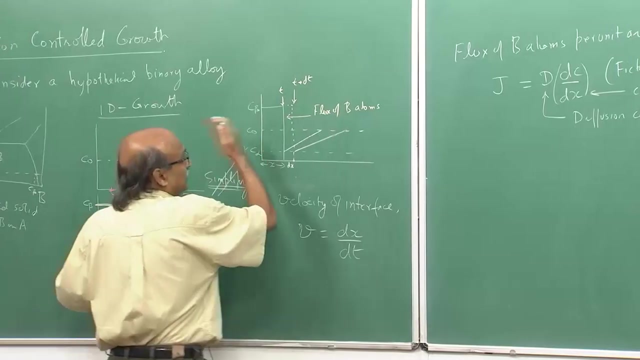 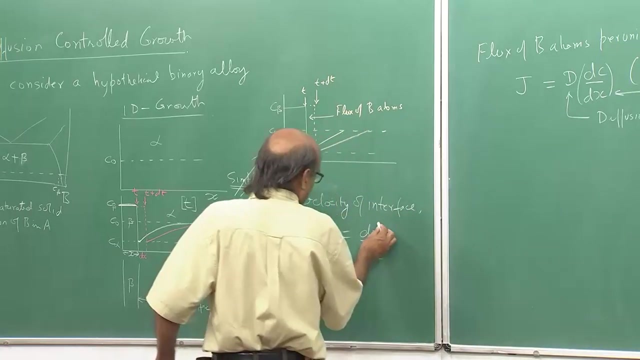 Which, in our simplified approach, if you look at this diagram, the concentration gradient is a constant because we have assumed a linear profile of concentration. So this is the rate at which B atoms are going to move per unit area, per unit time, The velocity of the 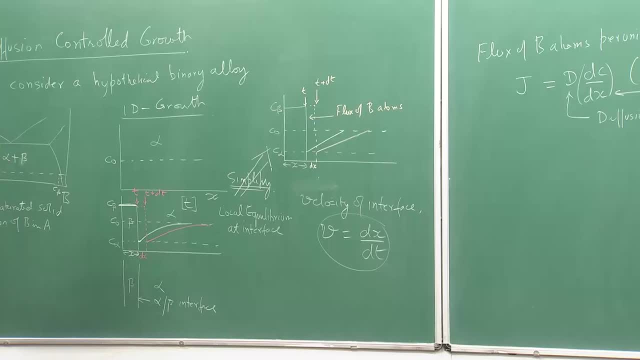 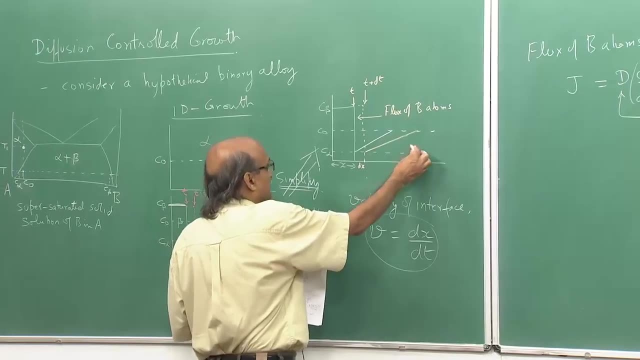 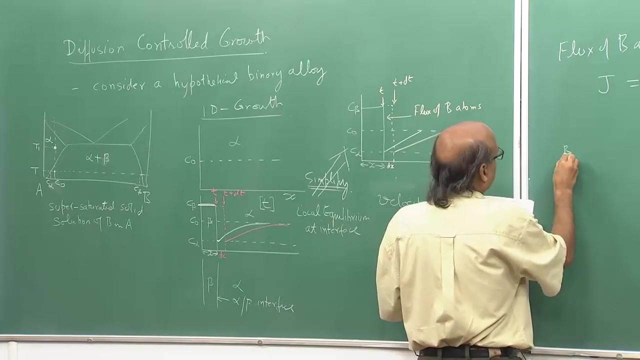 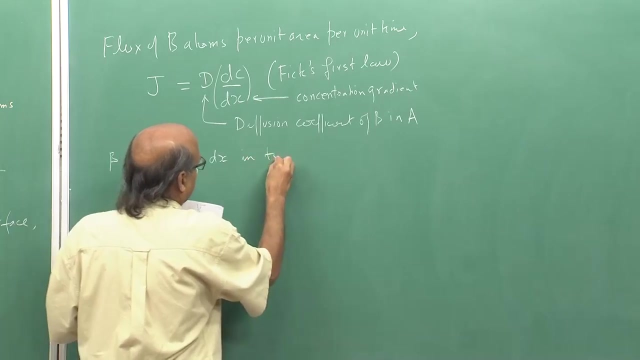 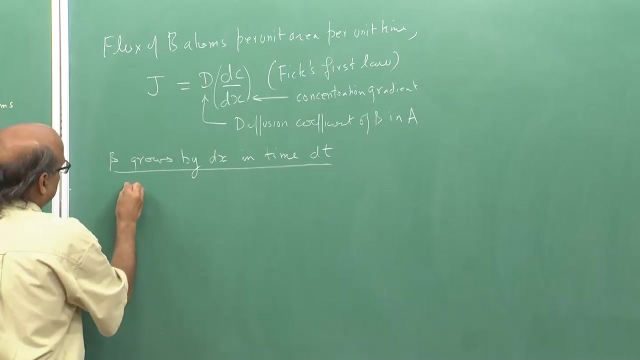 interface is d x by d t. So at what? At what rate? Essentially solute is getting added? B atoms are getting added to beta. So we say that beta grows by d x in time, d t. So then rate at which B atoms are getting. 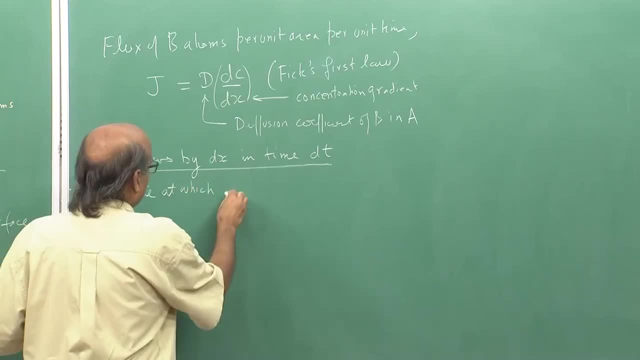 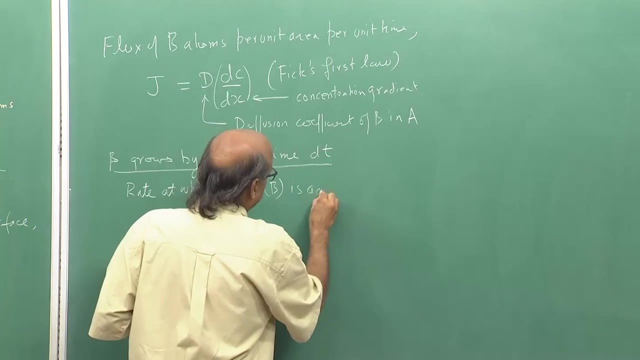 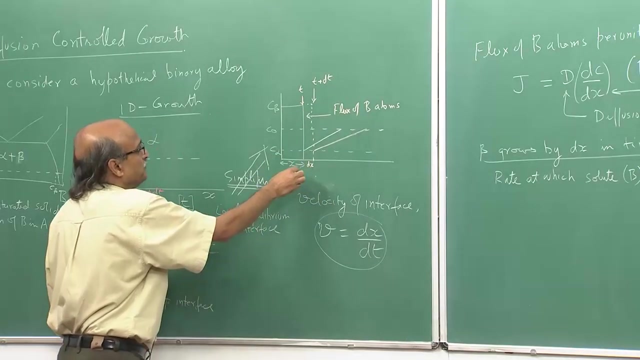 added Solute, that is, B atoms is added, is equal to well, look at the amount of B atoms that are added, which is nothing but C beta minus C alpha. So it is C beta minus alpha. So I have 1 minus 2 C beta. 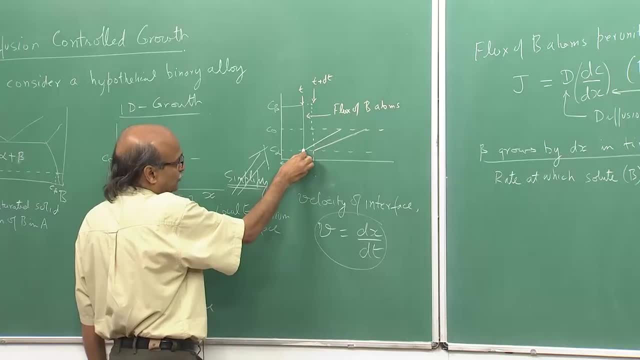 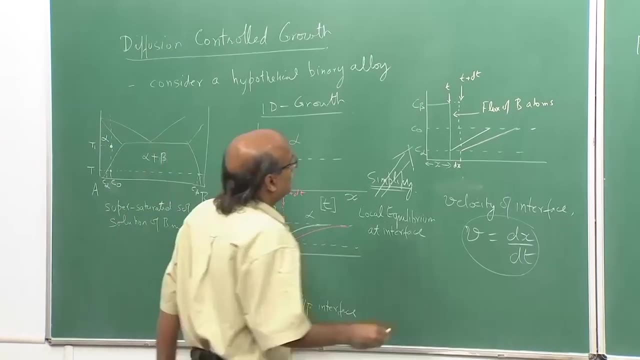 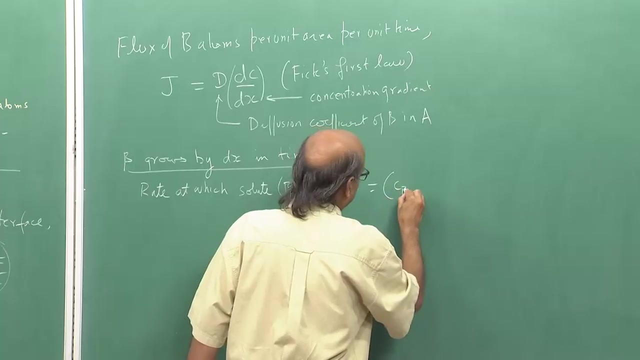 I have 1 minus 2 C beta. So I have 1 minus 2 C beta, So I have 1 minus 2 C beta here. the concentration of C alpha- this is this concentration you can think- is in terms of moles per unit volume, So C beta minus C alpha, multiplied by d x, by d t, So the 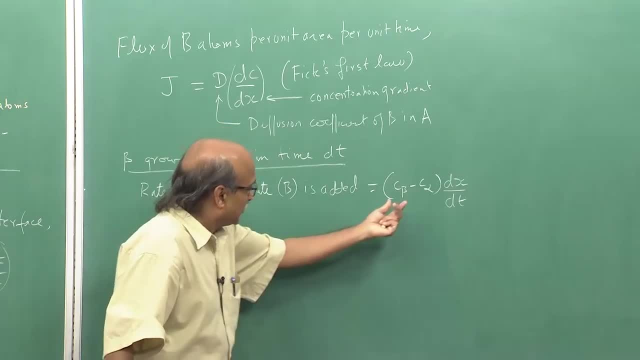 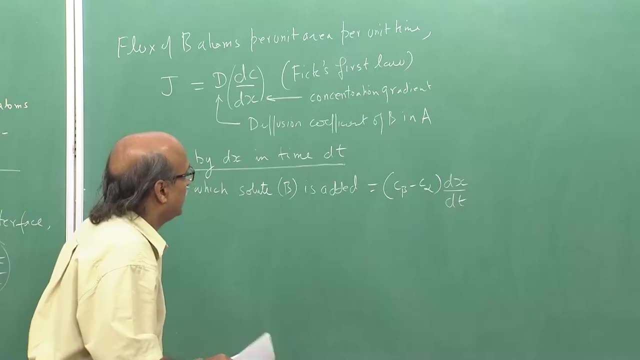 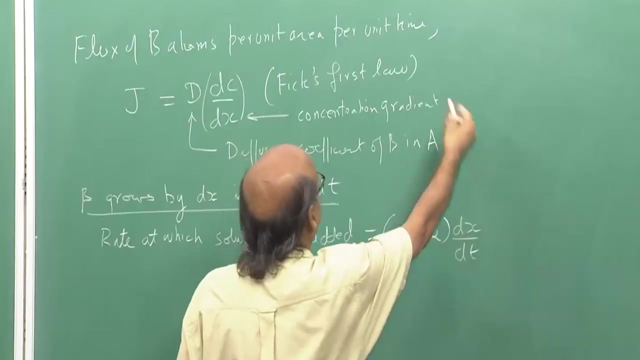 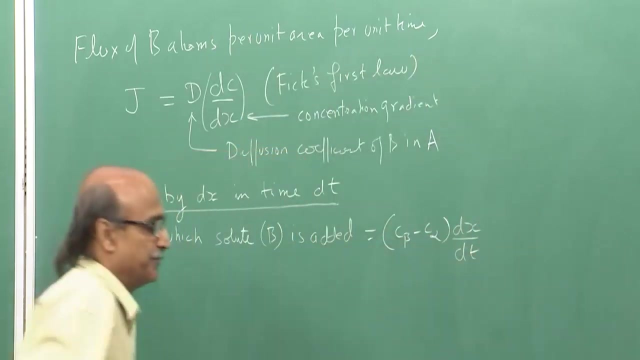 concentration, let us say, is in moles per unit volume, multiplied by the velocity of the interface, d x by d, t, and the units for this would simply be: would become, in terms of flux of B atoms in moles per unit area, per unit time. So this is the rate at which B atoms are getting. 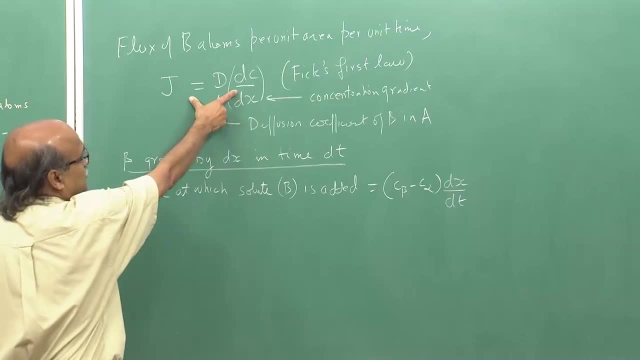 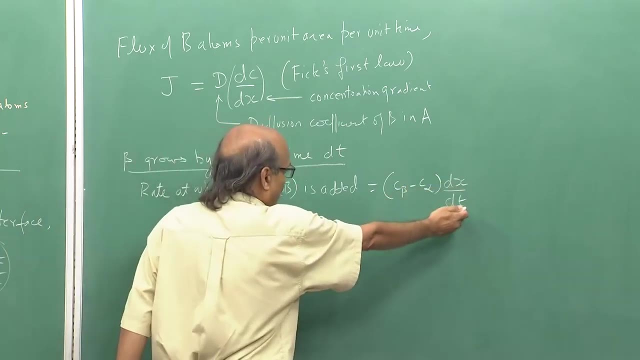 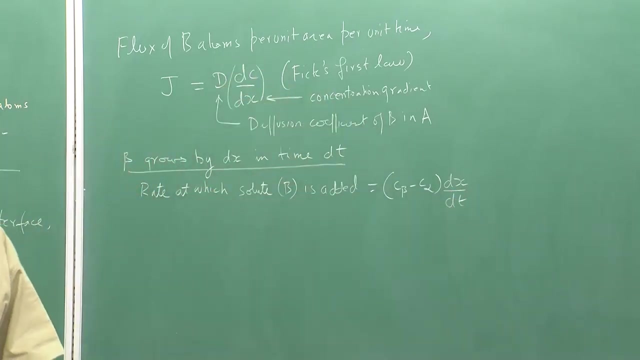 added: this is the rate at which B atoms are arriving at the interface and obviously the flux for this rate and for this velocity that two have to match, have to balance, And therefore I can simply write C beta minus C alpha, d, x by d t, to be equal to d d c by: 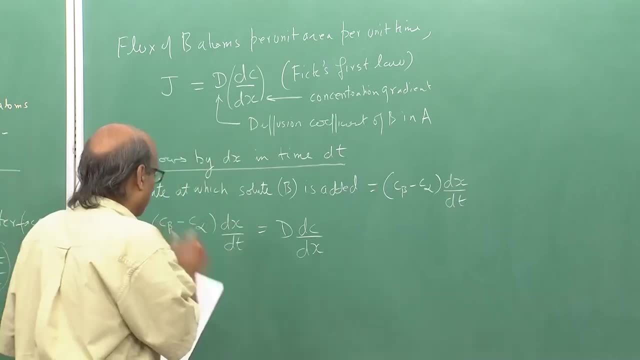 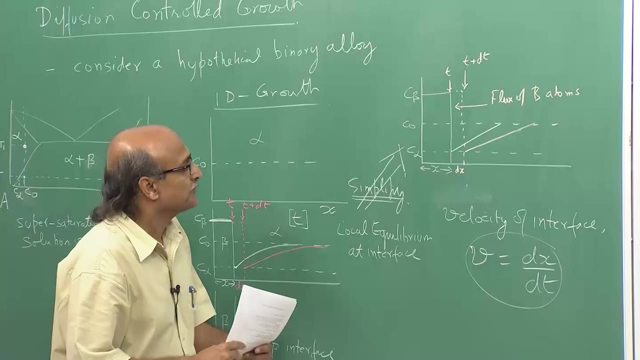 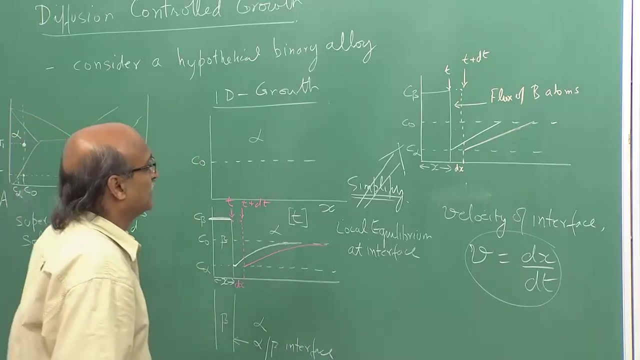 d x. Now let us look at it. what is d C by d x? If I go to my simplified representation here, d C by d x is a slope of this line, and that is nothing but C naught minus C, alpha divided. 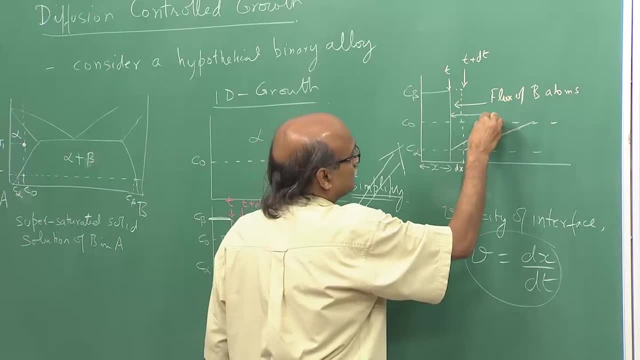 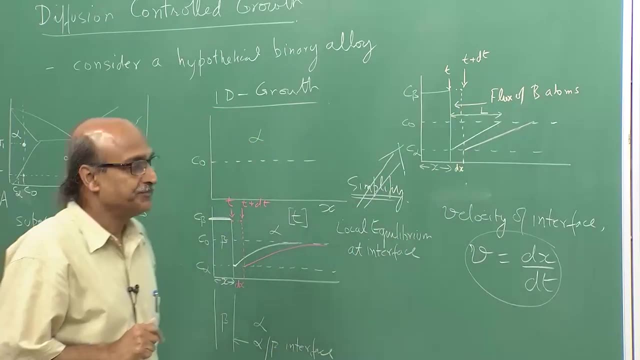 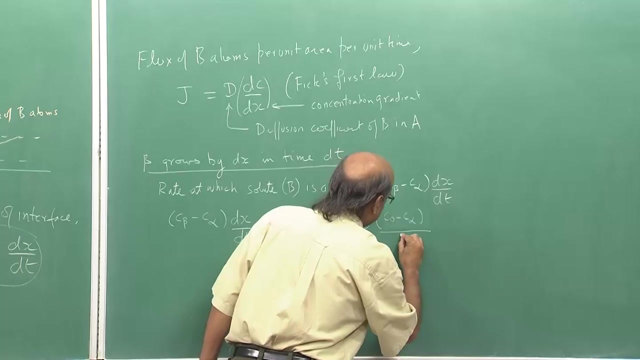 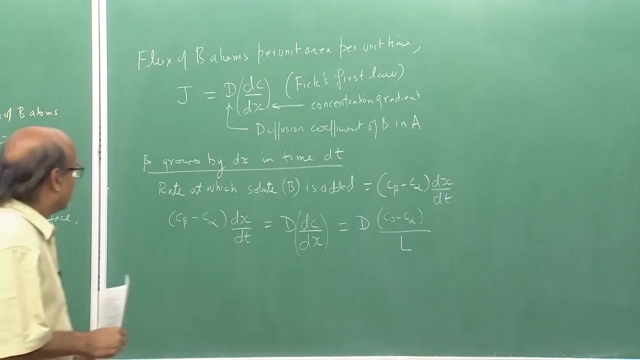 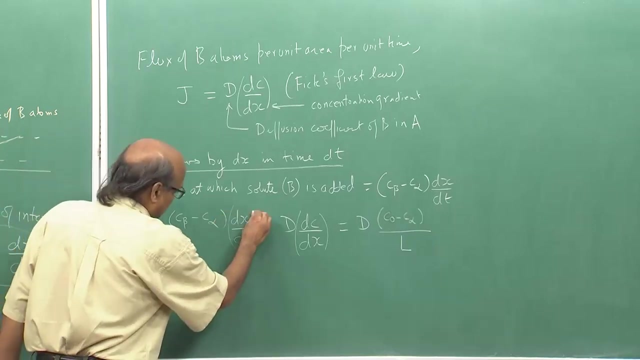 by some length, l ok. So I write this as d times divided by l. Ok, Ok. Now what do we do with this relationship we have? We wanted to find this, So this is a unknown quantity for us: C, beta, C, alpha. we know from the phase diagram, I know D, the. 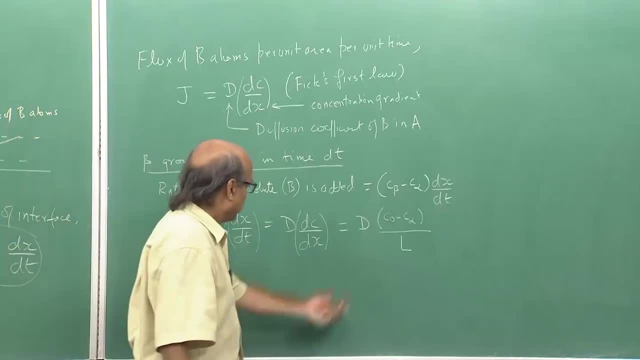 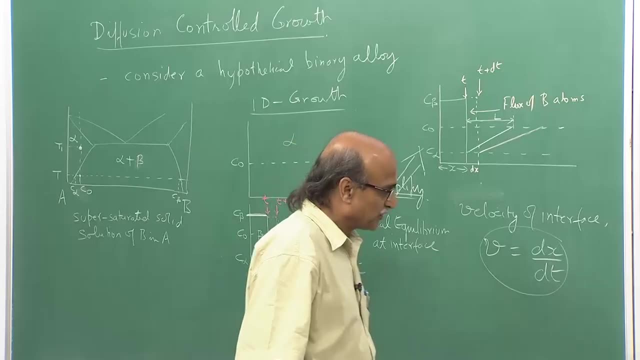 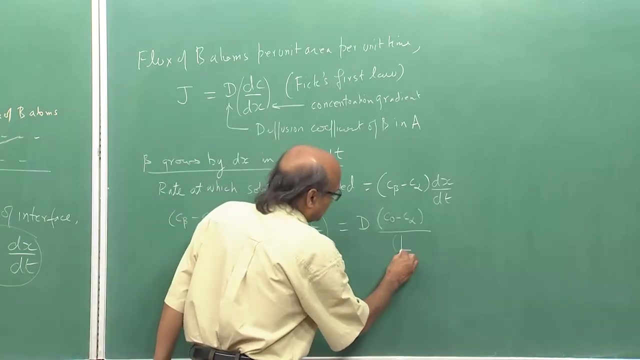 diffusion coefficient of B in A. I can get from there is a huge database of values of this diffusion coefficient D, or it can be obtained from experiment. So the other unknown quantity that is left is L. I do not know what is this distance. 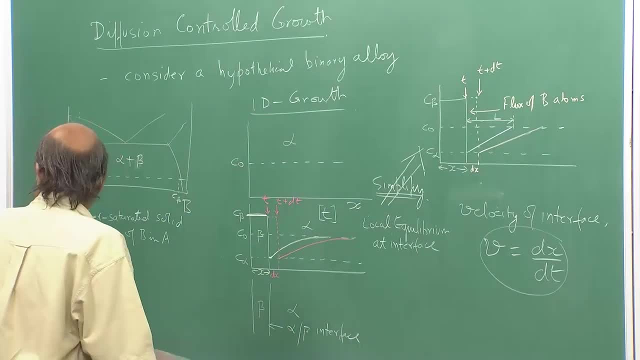 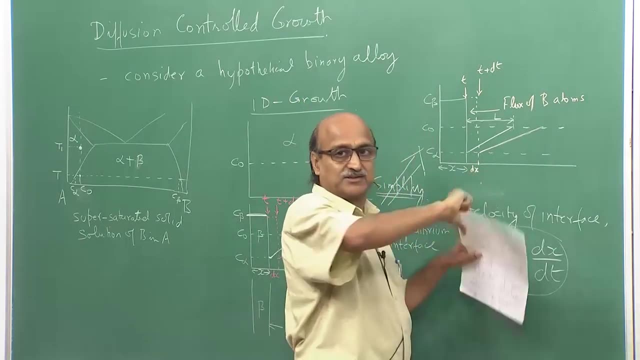 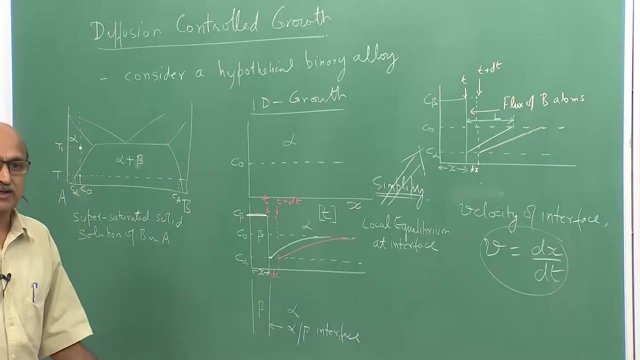 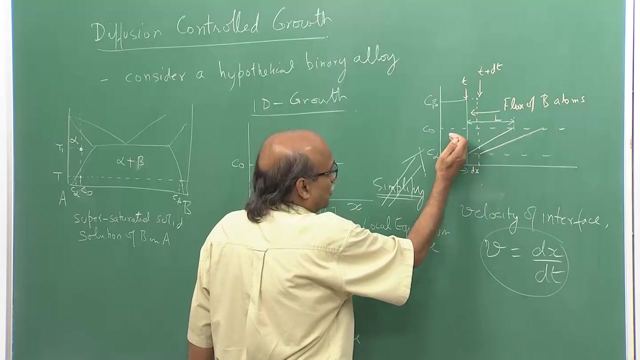 L How do I find this distance? L. Well, that is actually quite easy. In the system there are no atoms going out of the system, no atoms coming into the system. there has to be a mass balance. atoms are conserved. So if the concentration is increasing here, 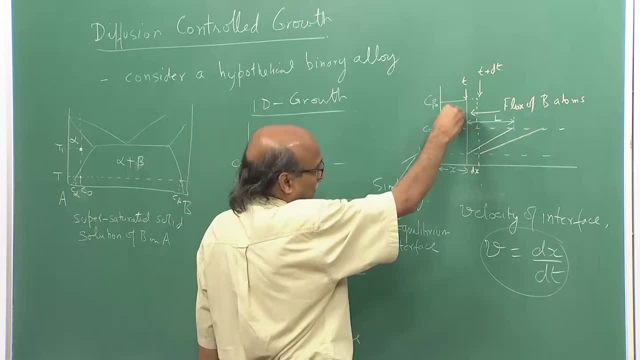 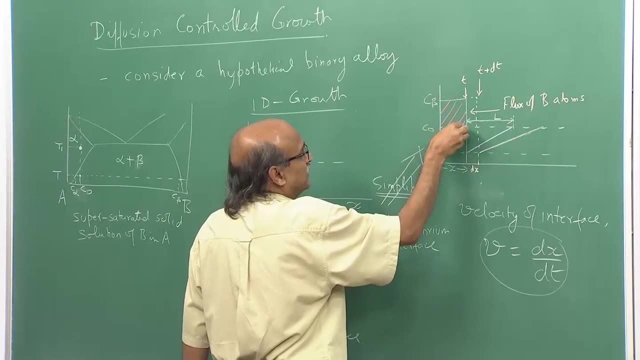 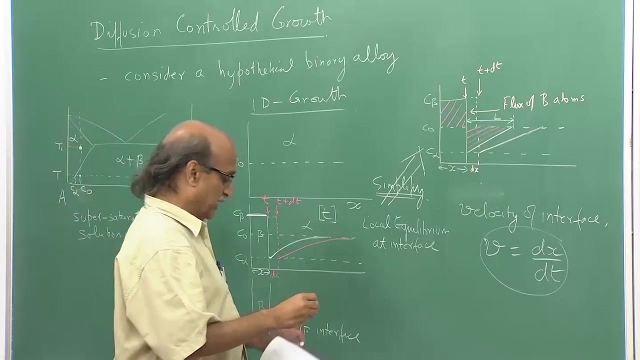 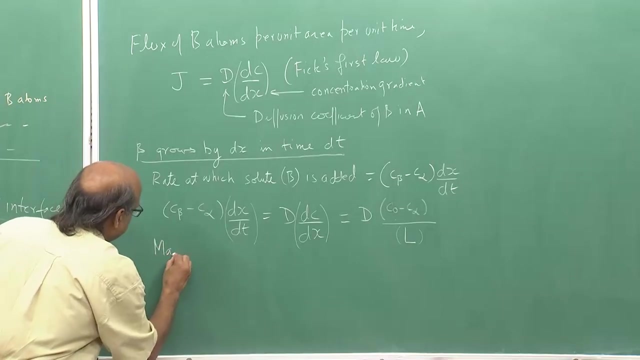 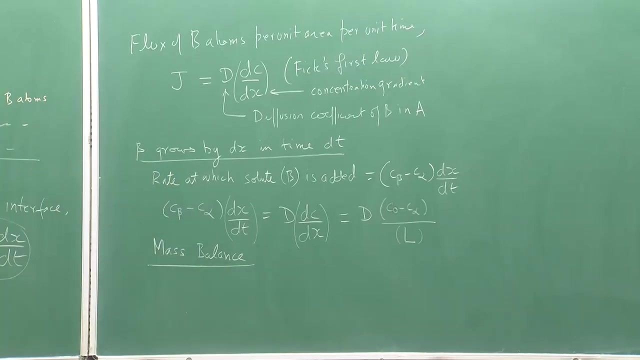 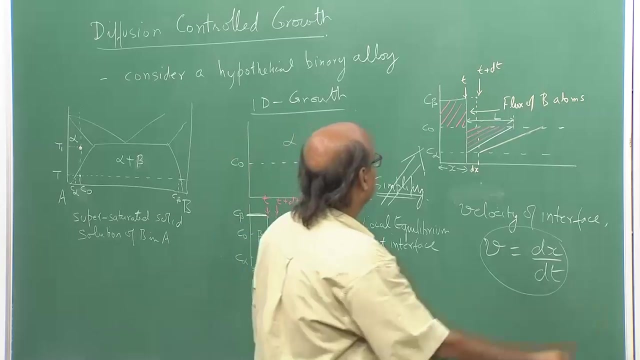 it is decreasing elsewhere and hence, if I look at this simple diagram, This area should be equal to this area for mass balance. So, from simple mass balance idea, the two areas are equal. So what is this area? This is simply a rectangle and this area is a mass. 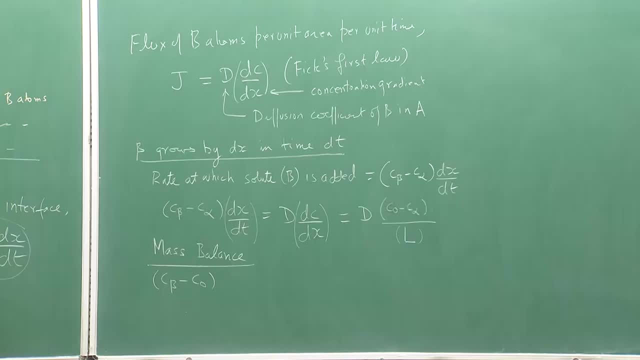 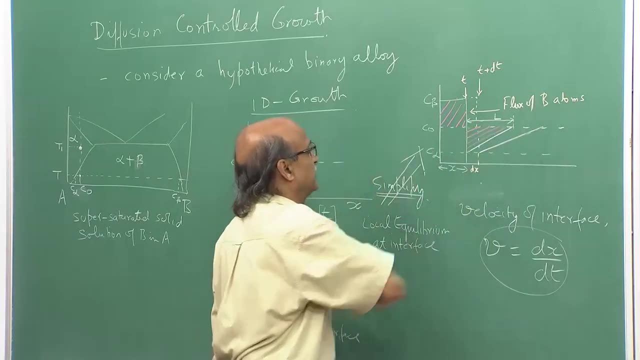 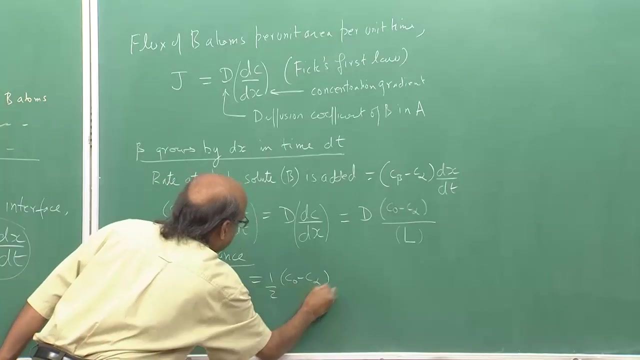 environment, Then another where what is going to happen in V theta is we have to solve this kind of calculation. If this is V theta, then we do not only do this, then we do not. and whether this complex equation takes place in this area, Now how do we find it is simply a thickness equation. 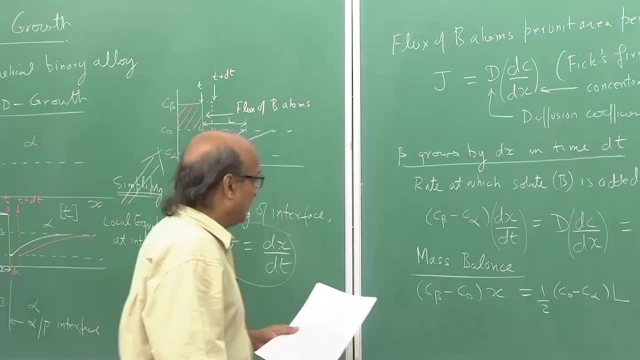 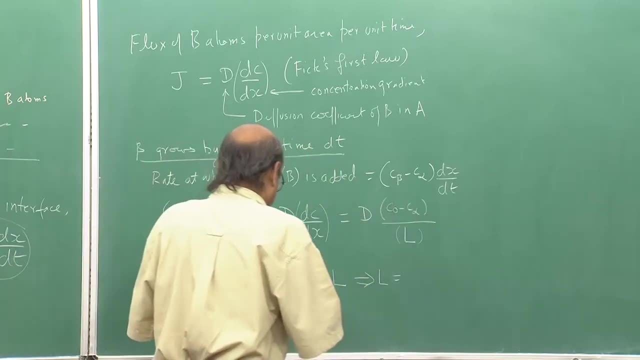 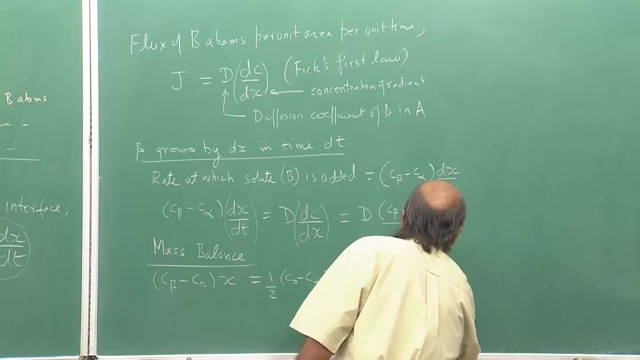 Our connection to the other vertical area. and then this growth is equal to the colour of L And the ornith Annual Alphameter is a well planed layer. We take different points, And that is simply rearranging the terms to c beta minus c naught divided by c naught. 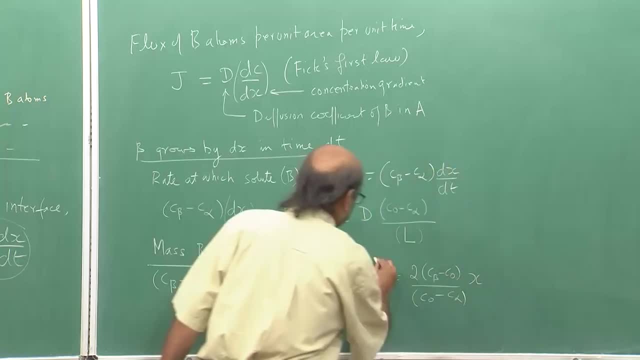 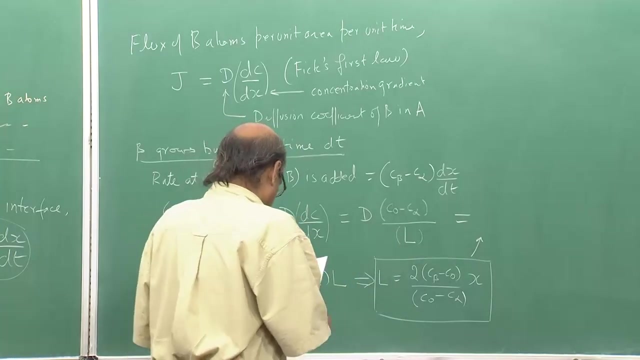 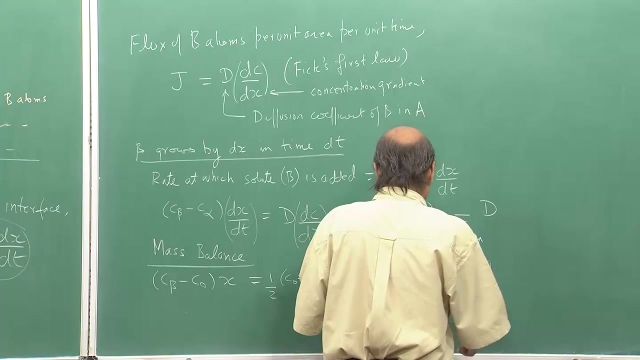 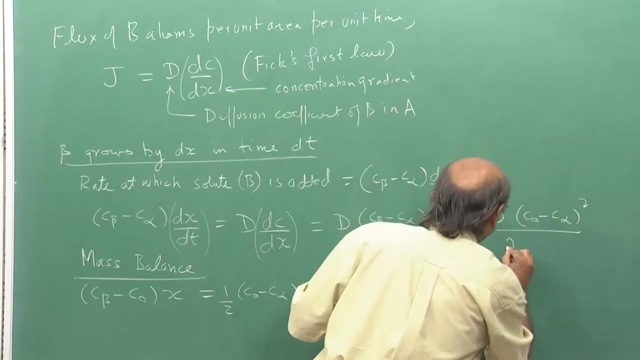 minus c alpha, multiplied by x. So this is the value of the unknown quantity L. So if I substitute this in this, I will get d times c naught minus c alpha, c naught minus c alpha square upon 2 c alpha. 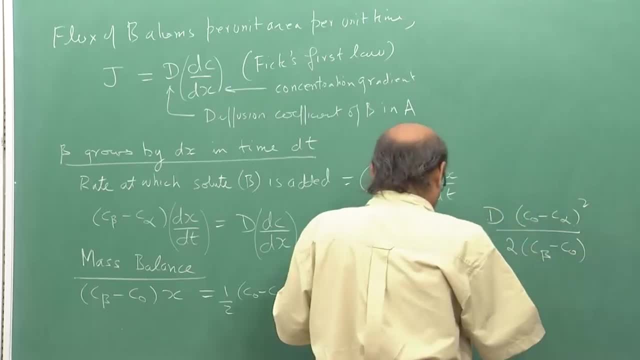 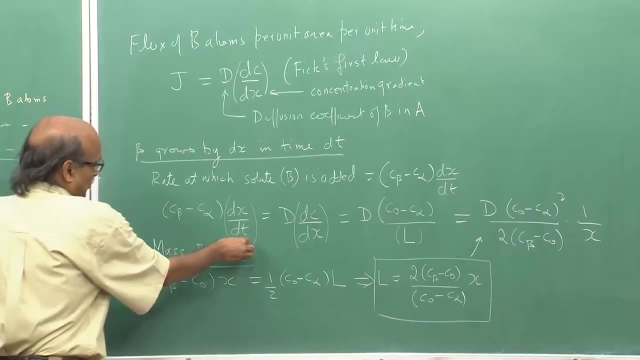 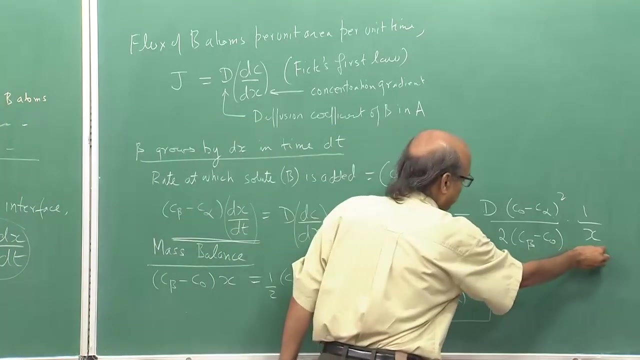 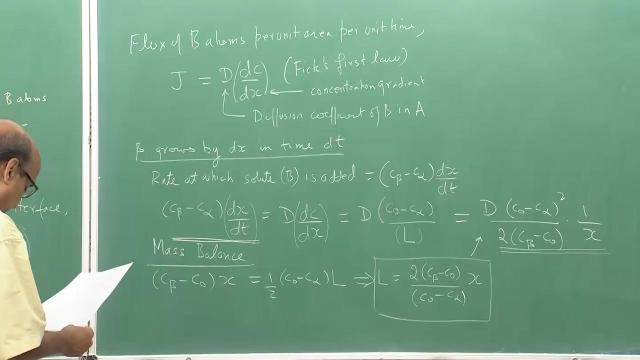 So c, beta minus c, naught times 1 upon x. So this is the rate at which solute atoms are getting added, and that is equal to this on the right hand side. Now this should be at. this, in fact, is a fairly easy quantity to solve, is a very simple. 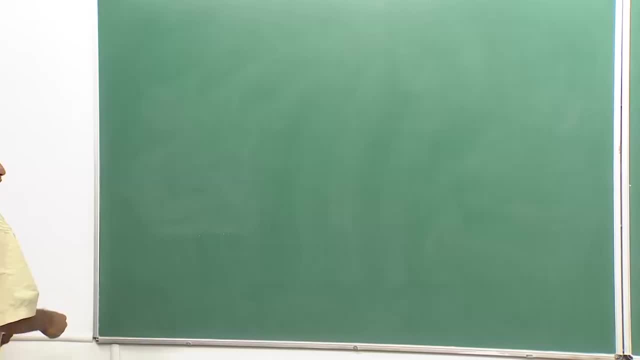 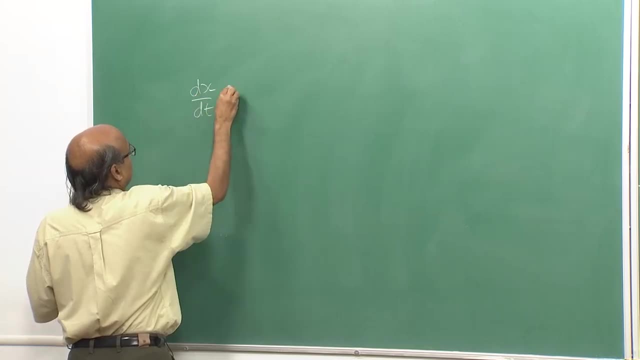 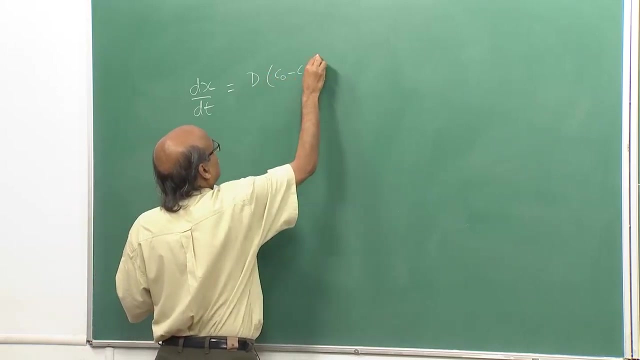 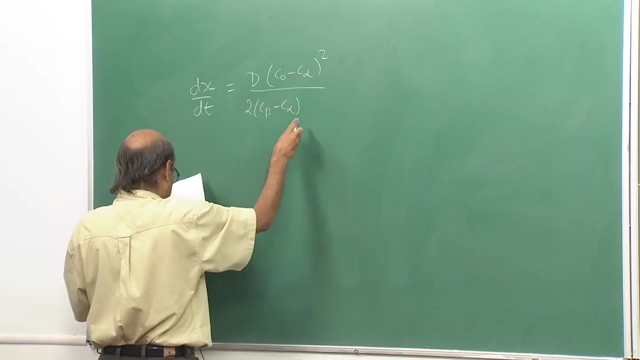 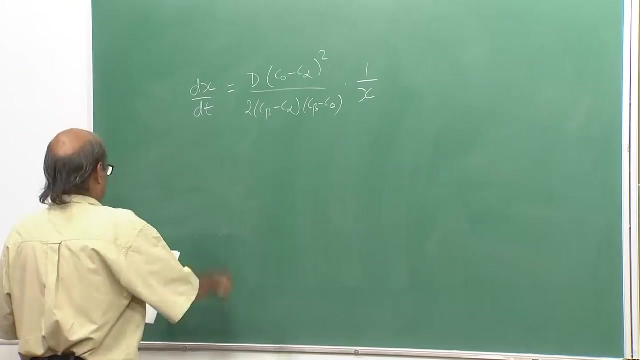 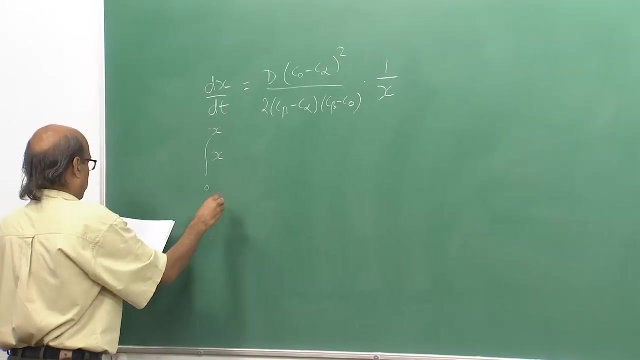 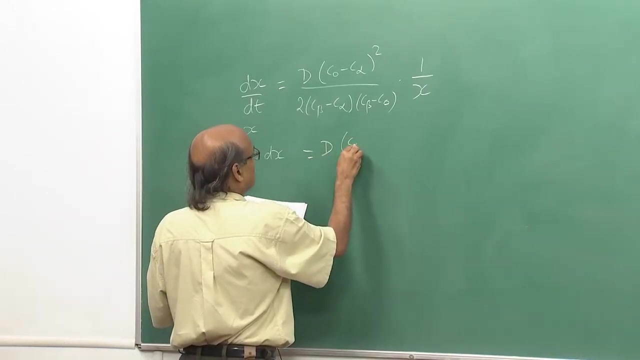 Differential equation. So let me rewrite this as: d: x by d t equals d times c naught minus c. alpha square upon 2 times c. beta minus c. alpha times c. beta minus c naught times 1 upon x. Solving this, integrating both sides: x: dx equals d times c naught minus. 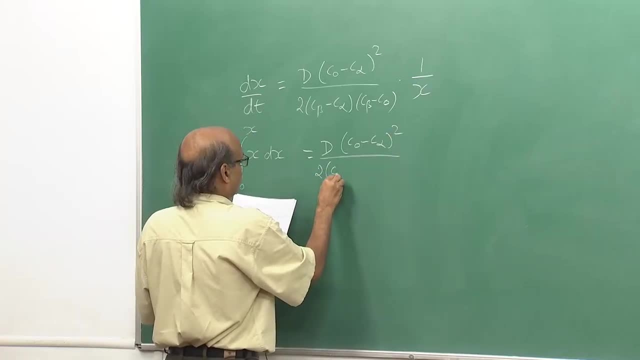 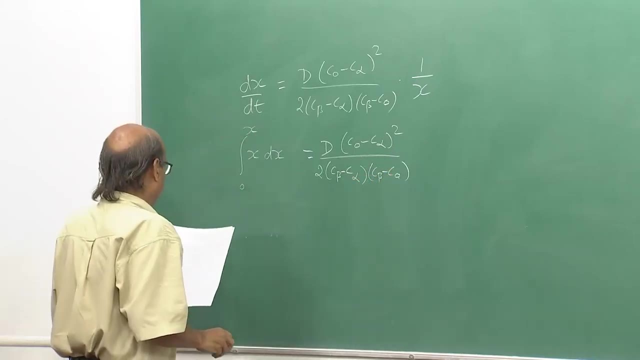 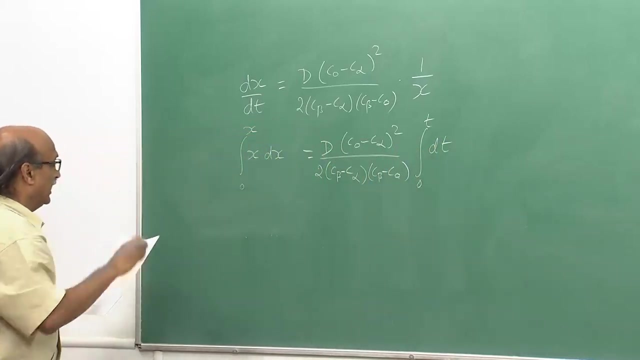 c alpha square upon 2 times c. beta minus c. alpha times c naught plus c alpha upon 2 t, So that is equal to 2 times c naught minus c. alpha square upon 2 times c beta minus c minus c. alpha times c. beta minus c naught 0 to t, dt, and this gives me x to be equal. 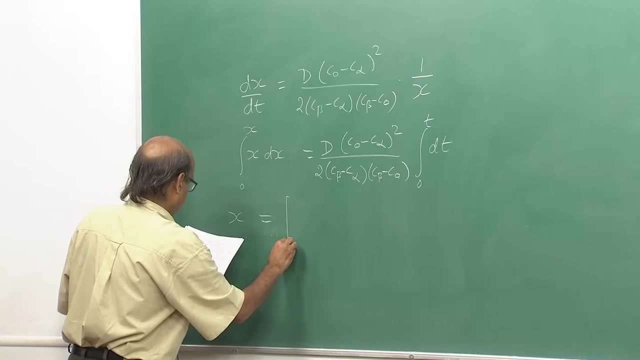 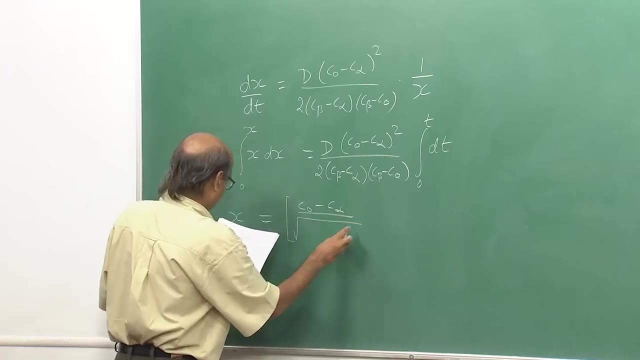 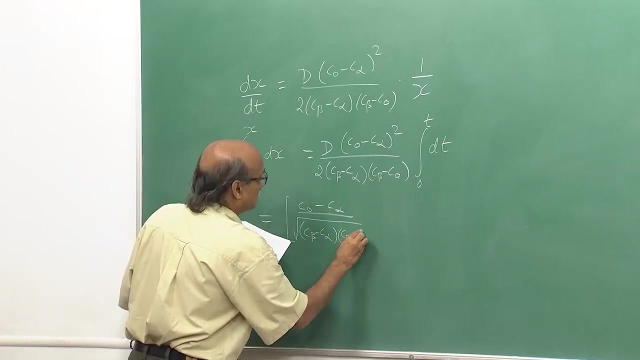 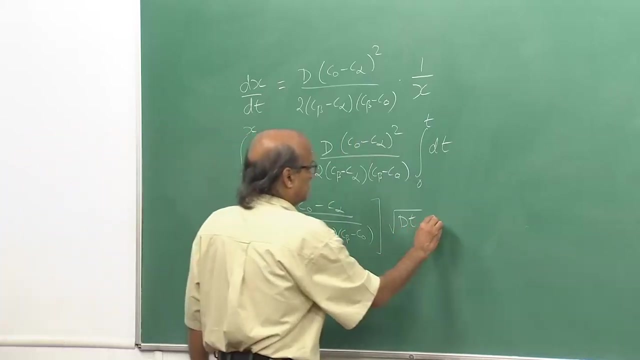 to c naught minus c, alpha upon square root of c beta minus c alpha times, c beta minus c naught. just simple rearrangement of terms, and this gives me how x varies as a function of time. So the interesting thing is this tells me that x is directly proportional to square. 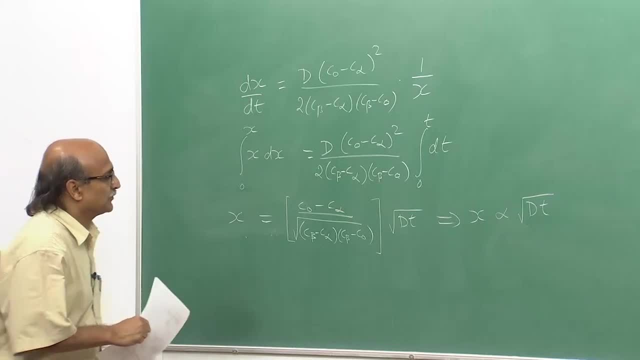 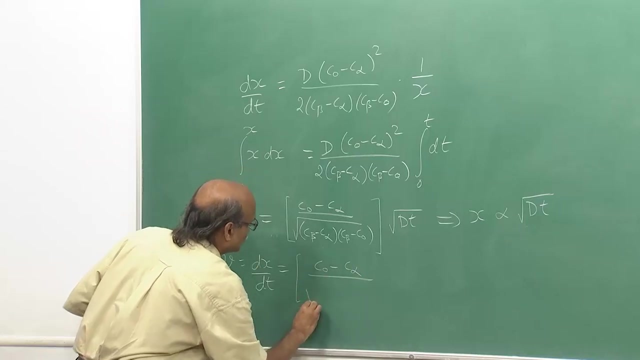 root of dt, where d is a diffusion coefficient and t is the time. And now, if I look at velocity, which is dx by dt, well, that would be same constant term, c naught minus c, alpha, On square root of c, beta minus c, alpha times, c, beta minus c naught square root of d by. 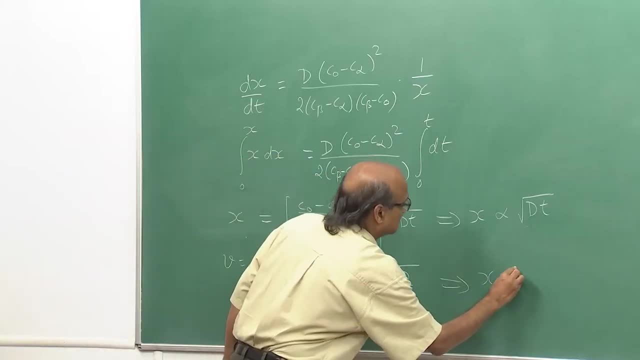 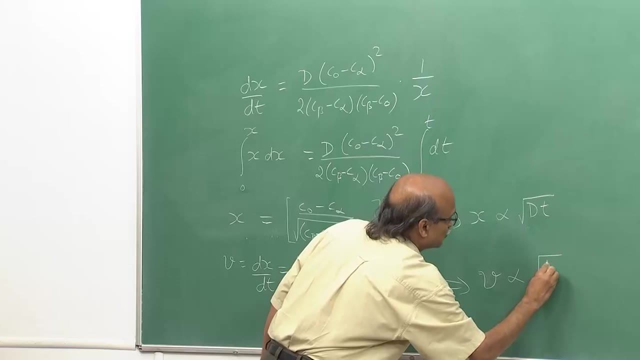 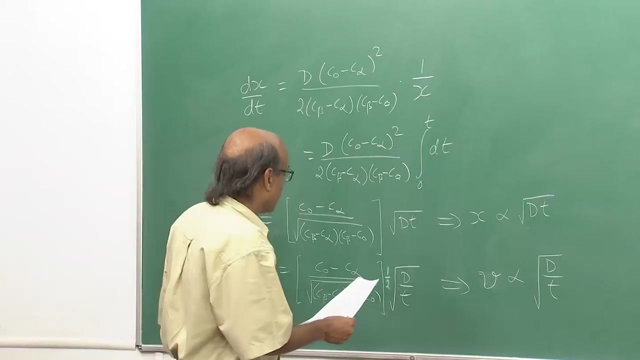 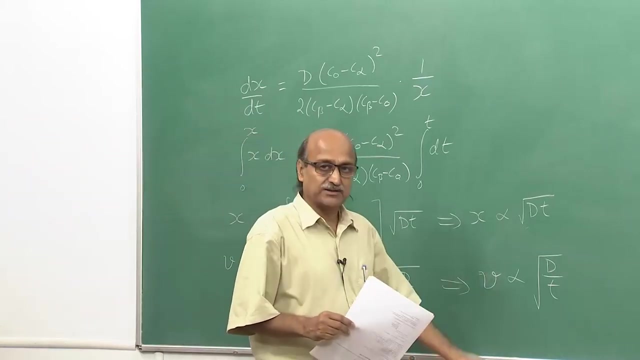 t, and that is simply that x is directly proportional to, not x, but the velocity v is directly proportional to square root of d by t. So one thing is clear: that growth rate is not a constant at a given temperature. in fact it is going to be a function of time. 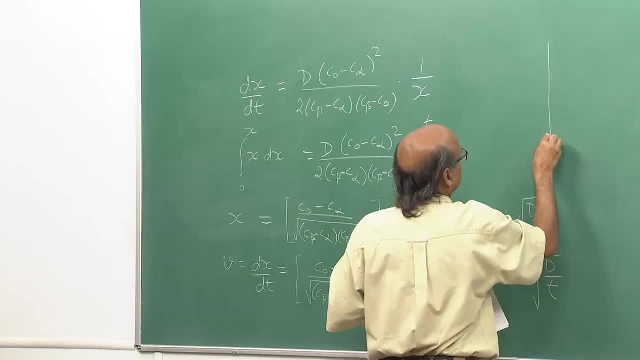 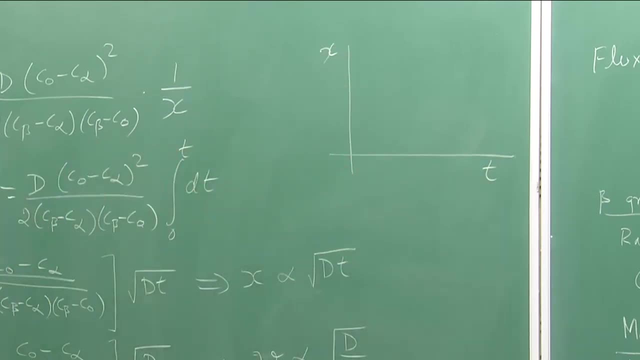 And if I plot, for example, x versus t, If I plot x versus t, I will get a curve like this. So, as growth is taking place, the rate at which growth is taking place is continuously reducing with time. So, in fact, points to note here are one: that growth is proportional to root dt and hence 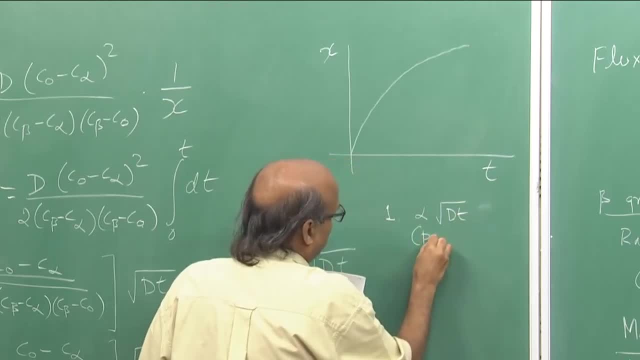 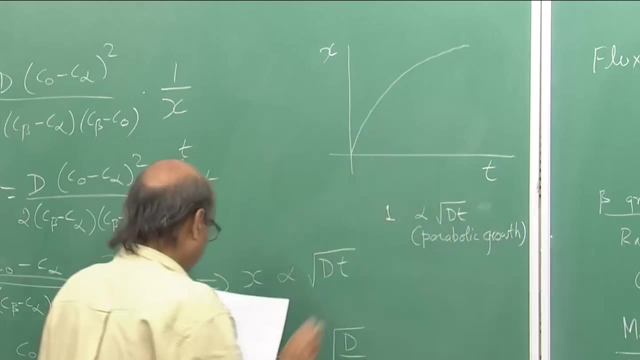 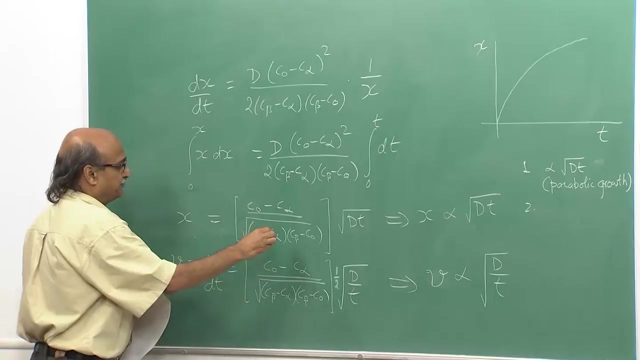 this is called parabolic growth to. if you look at this, c naught minus c alpha, this is super saturation. So if the alpha concentration was still c naught, So growth is proportional to super saturation. So higher the super saturation, higher is the rate of growth. 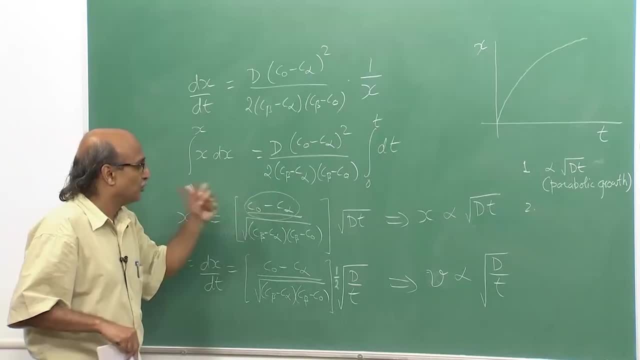 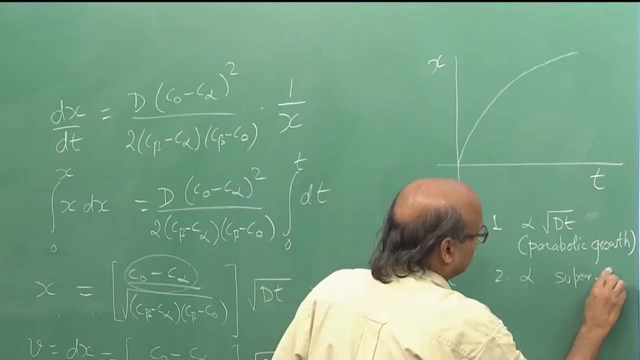 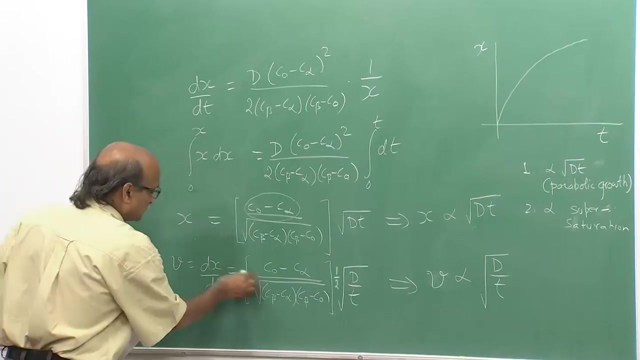 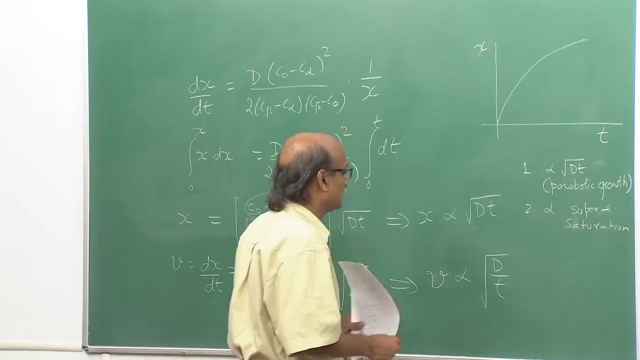 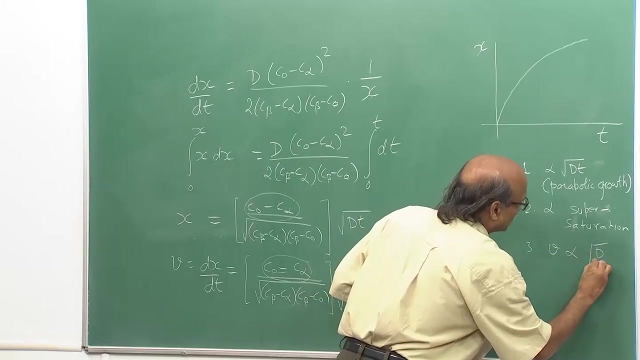 As you can see in the velocity also. 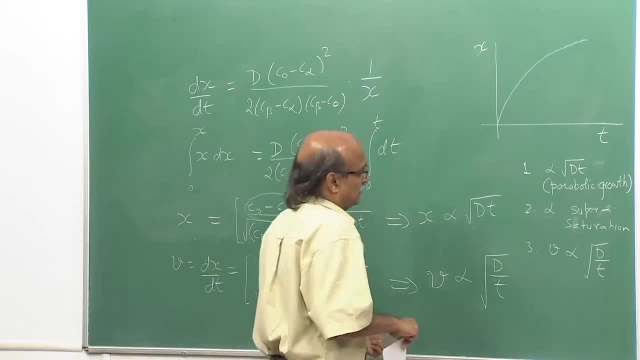 The velocity is also proportional to the root of would be peralion direction cut. 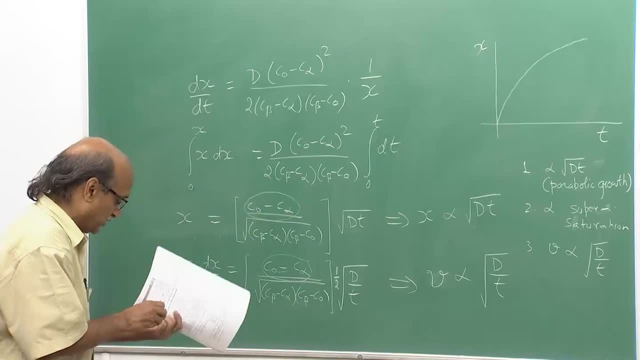 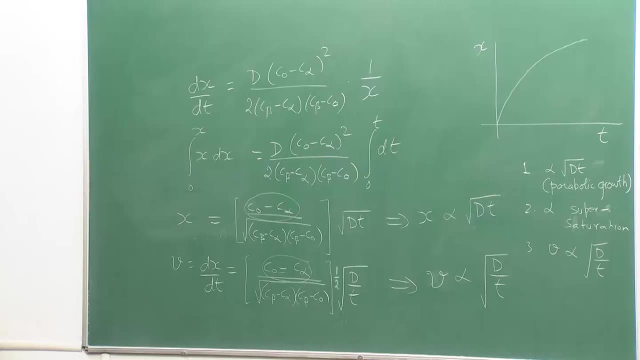 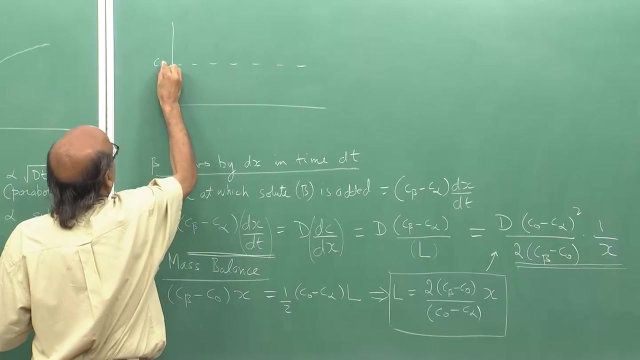 Now why is velocity reducing Of the growth rate is reducing with time? This could be understood if I very look at this choice level framework. You have to generate suchろ cetera with certain parameter for imagination diagram that as the beta precipitate is growing. So I have C naught, I have C alpha out here. 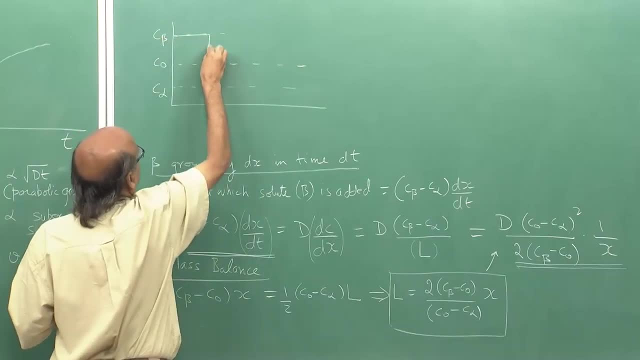 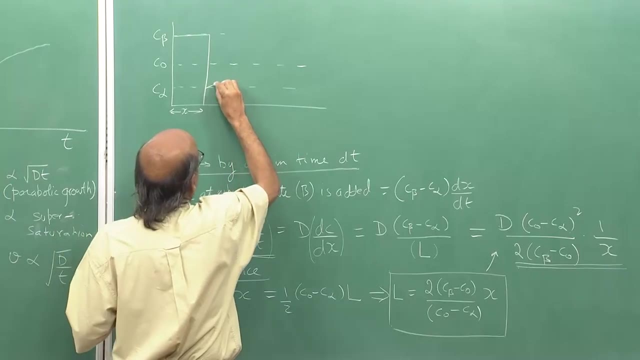 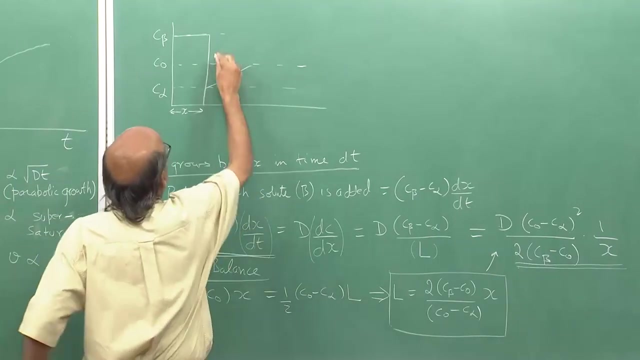 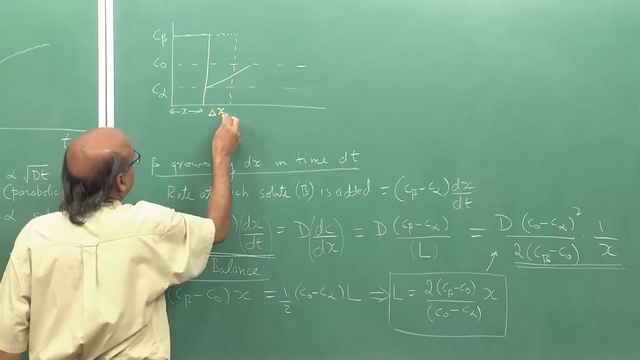 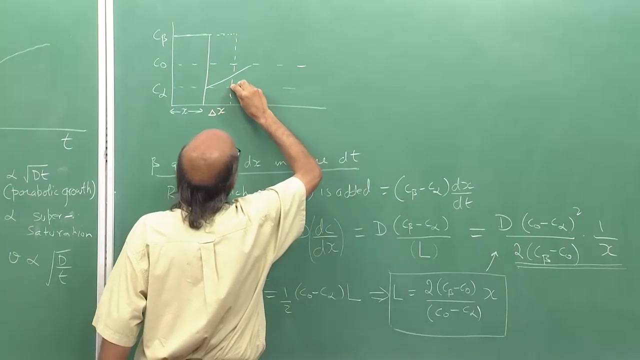 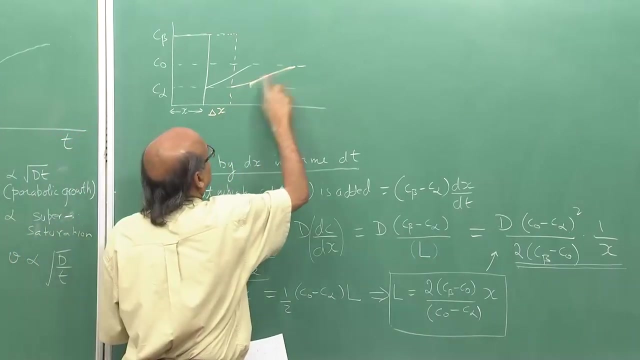 I have C beta- this is my beta- has grown by x and the concentration profile is this: Now, as growth takes place- let us say it is grown by delta x- the profile would become something like this: The slope- this is a straight line that the slope will. 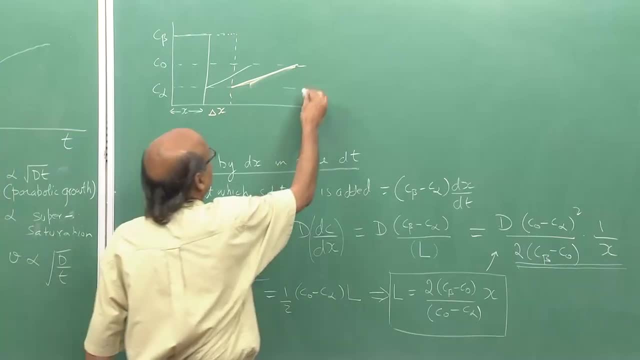 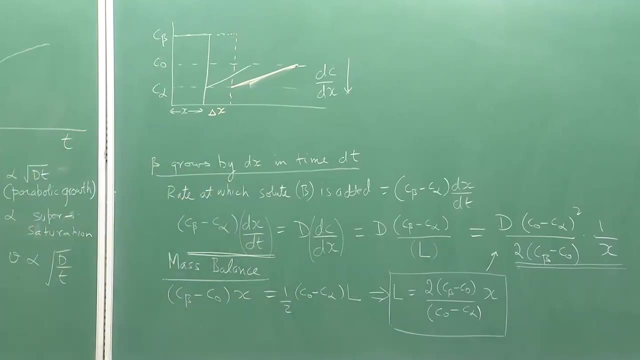 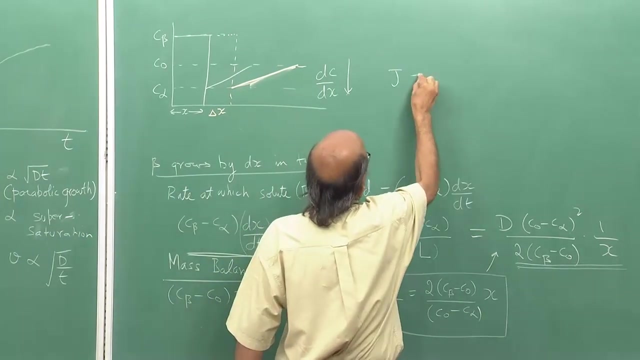 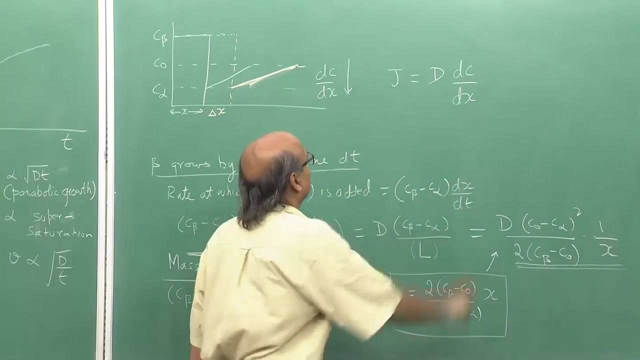 reduce. So that is d C by d x reduces with time, As d C by d x reduces with time. remember the flux which is given by diffusion coefficient times, the gradient of concentration. So as the gradient of concentration is reducing, the flux of B atoms are reducing.